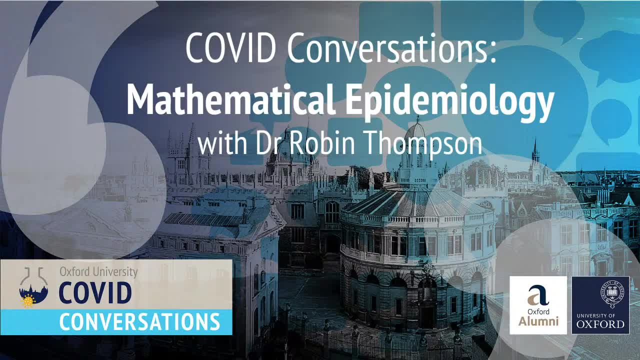 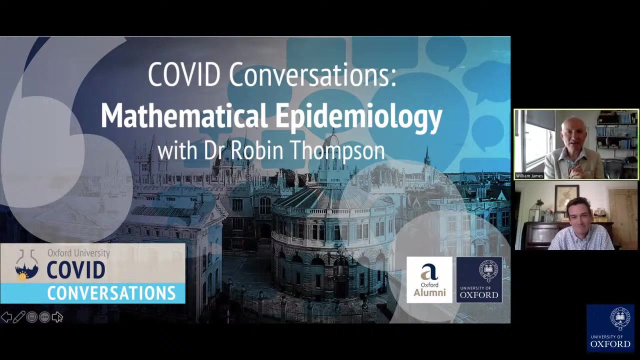 Thank you. Thank you, Welcome to the very final of a magnificent series of COVID conversations here from Oxford University. It's been a great series, but all good things come to an end And we're going to have an interesting talk from a mathematical biologist. My name is William. 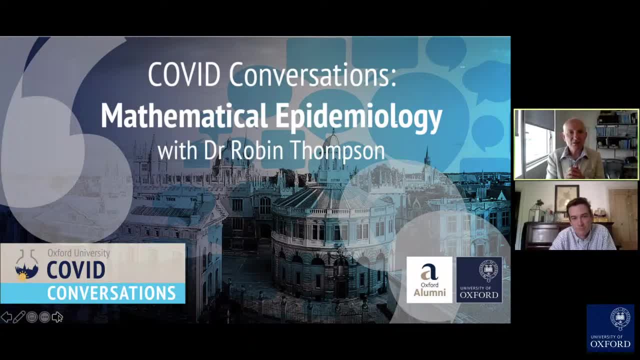 James. I'm Professor of Virology in the Sir William Dunn School of Pathology And, as you might have heard on some previous occasions, our containment lab does some of the core virology testing for the Oxford COVID-19 Research Network. It's my pleasure today to introduce 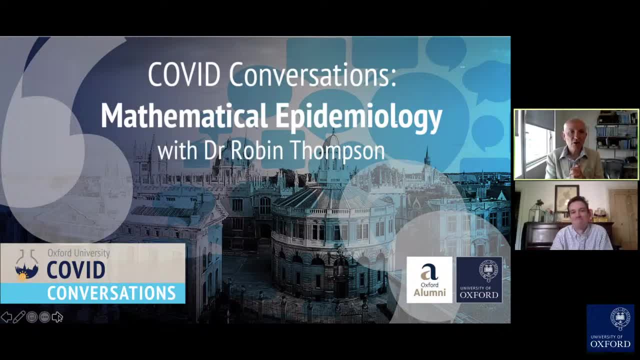 you to a junior research fellow at Christchurch, Robin Thompson, who's a mathematical biologist, who's been doing some of the really important work in analysing the epidemic and providing evidence and information to help guide responses to the way the epidemic has been developing and to try and control it in the most effective ways possible. So welcome to COVID conversations. 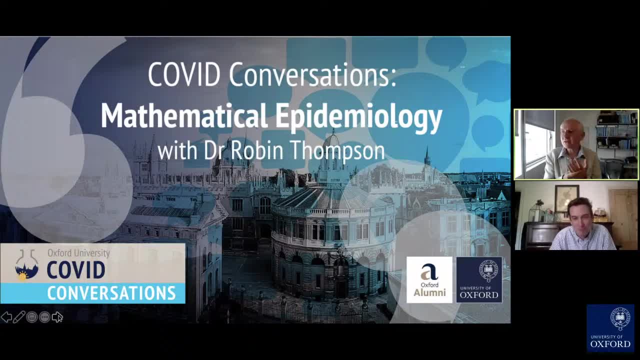 Robin, It's very good to have you here. I'd love to. well, before I kick off, I need to just say that you're going to be talking to us about 15 minutes and then we'll have some questions afterwards. And please, audience, we love your questions- If you could send your. 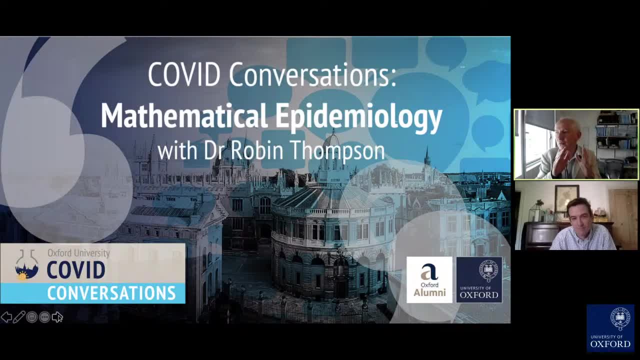 questions in through a chat window on YouTube or in the comments section on Facebook or any other linked social media. we will do our best to try and incorporate them into questions in the second part of the session. And the final note before we get going is: obviously, we're all working. 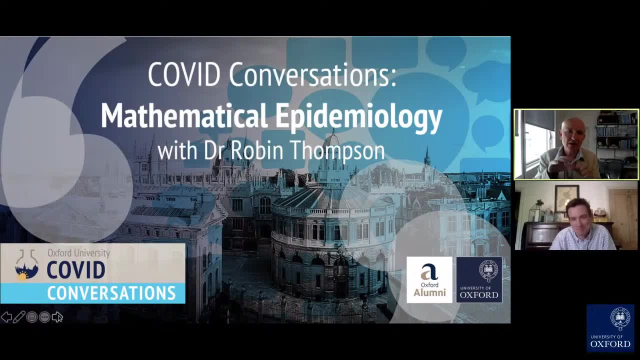 from different locations, not always with the best bandwidth possible, So there may be some glitches from time to time And I hope you just bear with us And you can always review the talk and the questions later on on YouTube. So with that out of the way, Robin, it's great to have you here. Of course, Oxford is. 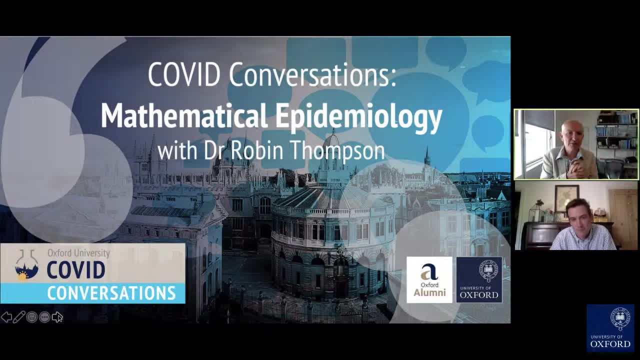 well known and it's one of the most powerful places I think on the planet has been for decades- in the whole applications of mathematics to biology and often in the epidemiology and infectious disease area. So thank you very much for joining us. 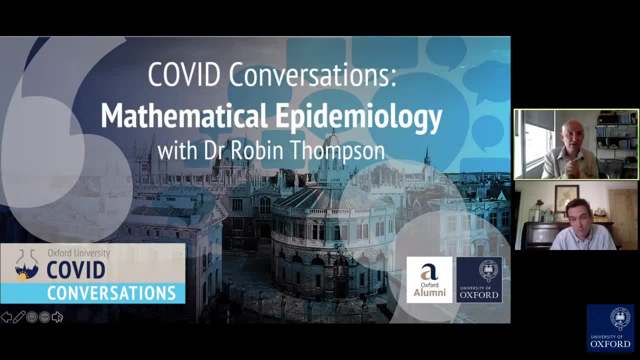 Robin Cigney, PhD, PhD. Well, thanks, Nick. So I'm going to the right section. I'll just come in and talk to you, But I'm going to be at the edge of my seat. I'll start by asking a question. 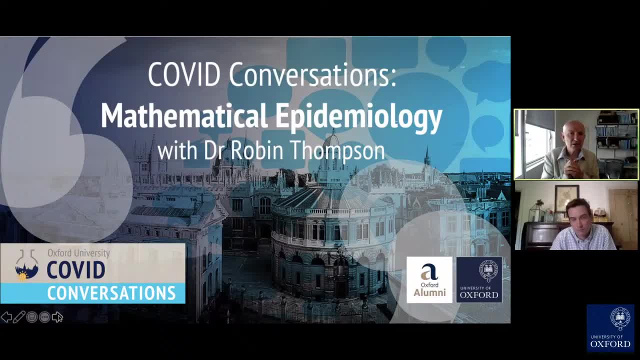 that I'm curious about, which is: is there a certain sort ofpción and expression that you think that the important needs of mathematics have, and what you're trying to achieve in a given area? I mean, that's a really important tradition that you're in there, And now is a 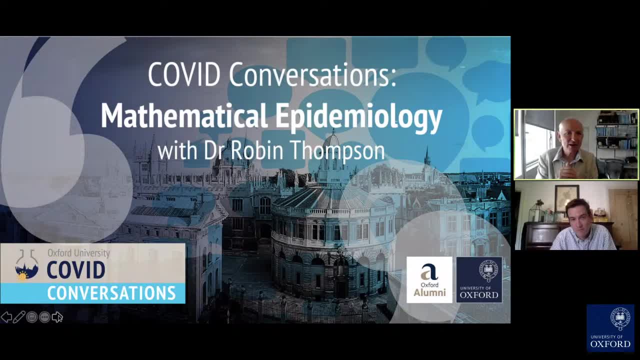 really good time for mathematical biologists to show how useful they are to us in the rest of society. Maybe we'll get people out there really interested in taking mathematics seriously as a applied subject, not just as a sort of puzzle thing for fun- although it is fun as well. 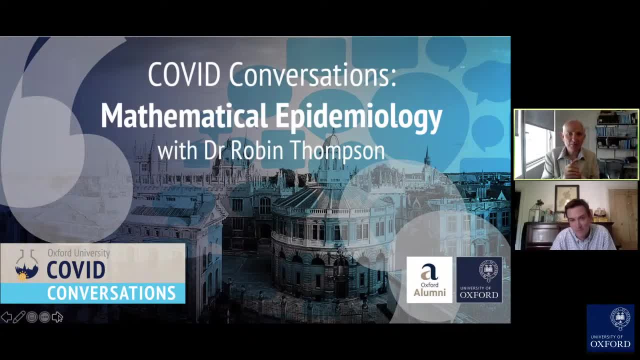 Before you start your talk, I'd love to pass you a question. I've been a student here for six years. Before you start your talk, I'd love to pass you a question I've been asked on several occasions. I make up an answer and I'm not a mathematician. I don't think it's necessarily a very good one. 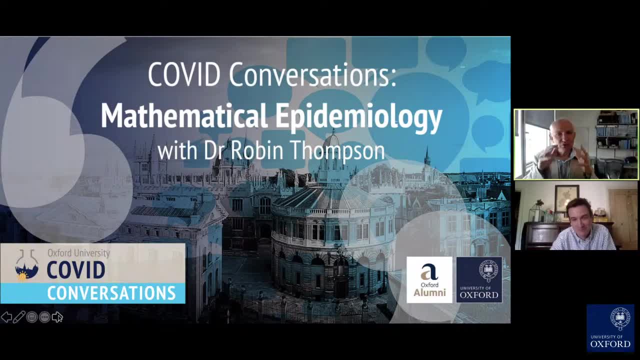 It's the R value. We're always hearing about R0 or R this, that or the other, and yet it's, as far as we can see, it's not something you can directly observe. So how on earth can they tell us today that the R number in Britain is 0.7 to 0.9?? How can they make that estimate? Perhaps you could kick off with a brief introduction to that. 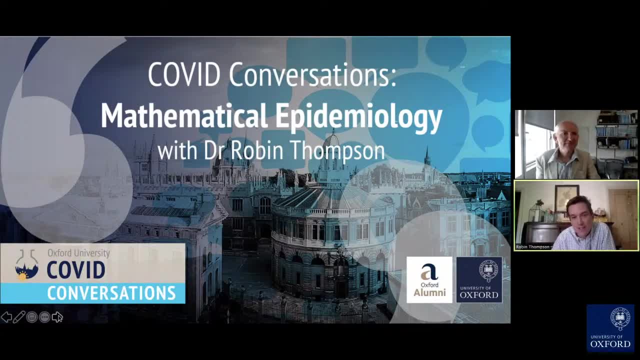 Yeah, sure. So, as part of the talk, one of the things that I'm going to do is actually take you through precisely one way of calculating the R number. The way it works in terms of the government estimate of 0.7 to 0.9, is that lots of different research groups around the country are asked to estimate the R number using slightly different methods. 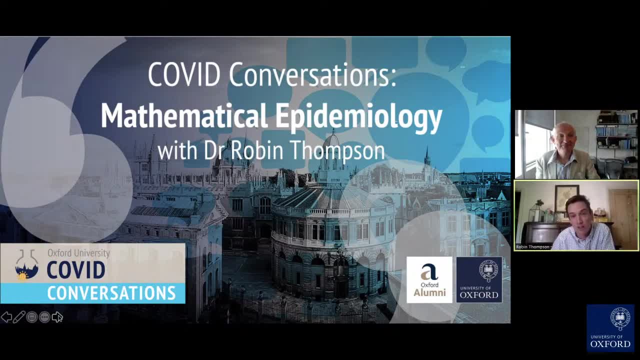 I'm going to describe one of those now. but what 0.7 to 0.9 reflects is that kind of range of different R numbers from different Like hole-of-hole sort of thing. yeah, Yeah, exactly, And lots of the methods are kind of similar but some of them are a bit different, but broadly they're all consistent. They all lie more or less in that quite tight range. 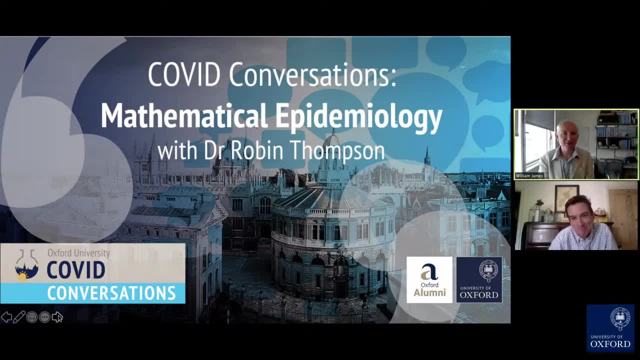 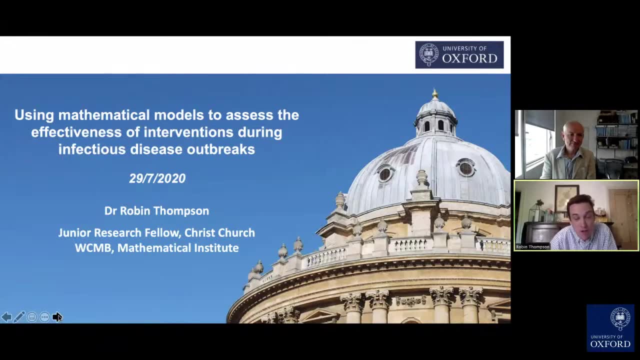 Excellent. Well, I think we're all looking forward to hearing how it's really done by professionals. Thank you very much, Robin Go away. Thanks very much. Thanks, William. Yeah, so, as you just heard, my name is Robin. I'm a junior research fellow at Christchurch and I work in the Wolfson Centre for Mathematical Biology in the Mathematical Institute here in Oxford. 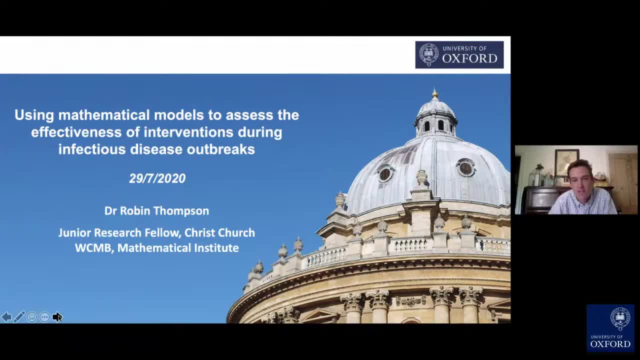 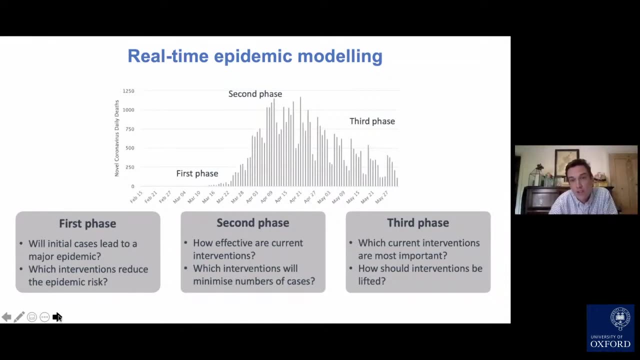 I'm going to talk about using models to assess the effectiveness of interventions during infectious disease outbreaks and, in particular, estimating the R number. So I'll come to that a little bit later in the talk. But broadly, the field of real-time epidemic modelling is all about using mathematical models to answer important questions at different stages of an infectious disease outbreak. 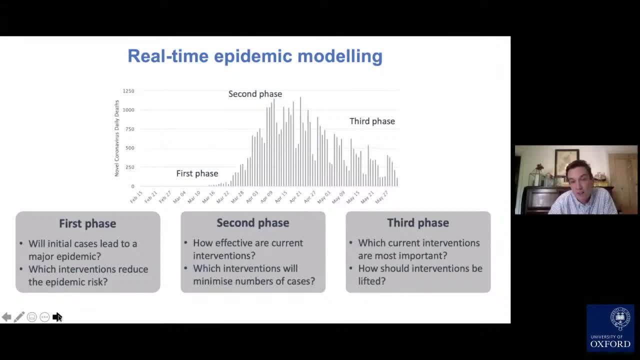 And as an outbreak goes on, the questions that we're interested in answering change substantially. So in the initial phase of an outbreak- which I guess was where we were back in January for COVID-19,, when we have very small numbers of cases, we're interested in answering questions like 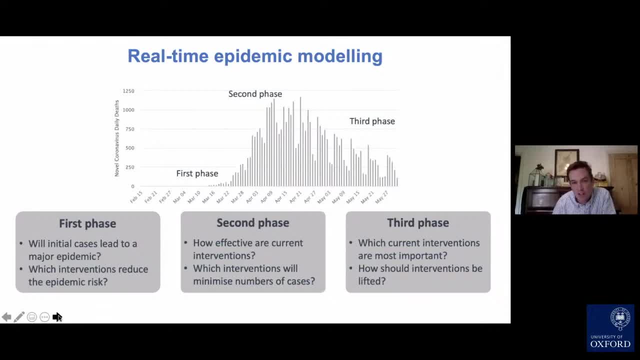 are those initial cases going to? Are those initial cases going to go on and spark a really large epidemic, or are they simply going to fade out as a minor outbreak At that stage? we're also interested in answering questions like: which interventions can we bring in to reduce the risk of a really large epidemic or, at the very least, to delay a really large epidemic? 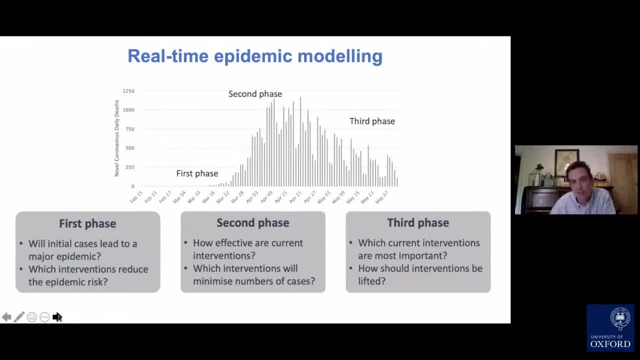 In the second phase of an outbreak, so when case numbers have started to increase and we know that we've got a major epidemic. we're interested in questions like how effective are current interventions, And that's where the R number comes in. The R number is sort of an estimate of how effective interventions that are in place at the moment are. 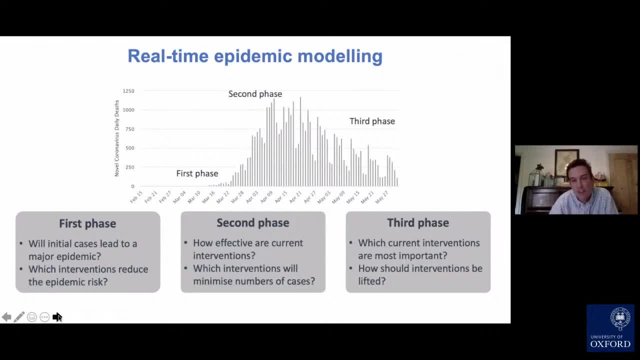 And we're also interested in questions like: which interventions can we bring in to minimise case numbers, or to minimise the numbers of deaths, or perhaps to keep the number of individuals requiring intensive care unit beds below the capacity? And then, if an infectious disease epidemic peaks and we're in the third phase, so cases are coming down again. 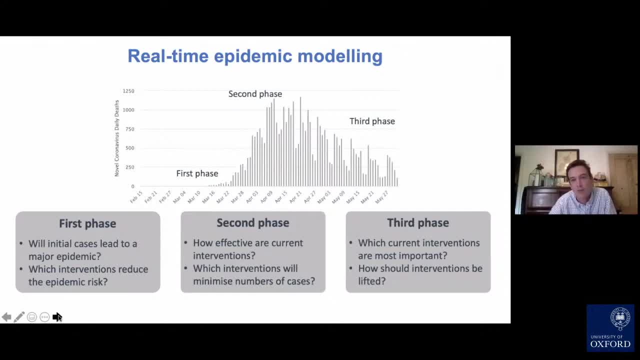 then we're interested in questions like which interventions can we bring in to minimize case numbers or to minimize the numbers of deaths? And then we're interested in questions like which current interventions are most important. Which of the current interventions are the ones that are sort of most integral to driving that decline in cases? 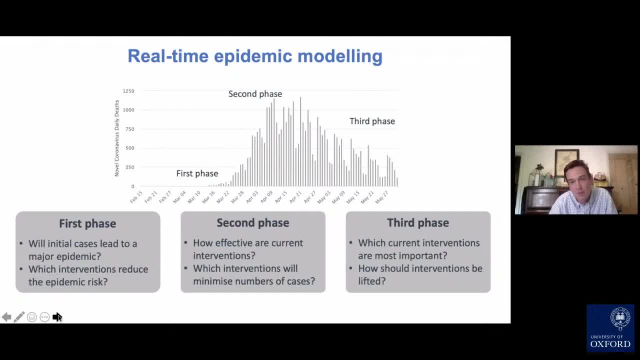 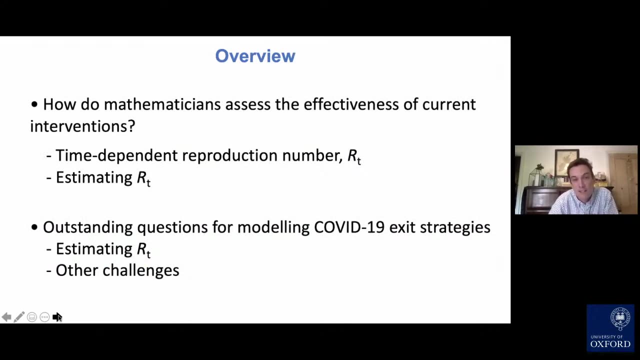 And then, related to that question, are there any interventions that perhaps are less important and can be lifted safely without risking perhaps a surge in cases going forwards? So, like I said, I'm going to focus in on one of those questions and, in particular, assessing the effectiveness of current interventions and assessing the time dependent reproduction number. 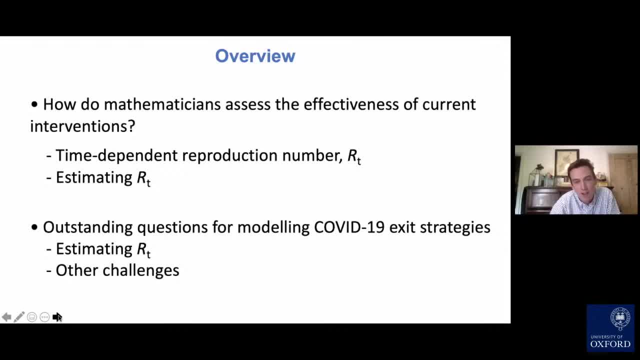 or R number. So this is the R number. I'd just like to give a flavour in this talk about exactly how the R number is estimated, In fact one particular method for estimating the R number. there are a few different approaches, And then at the end of the talk I'm going to go into a few outstanding questions for modelling COVID-19 exit strategies. 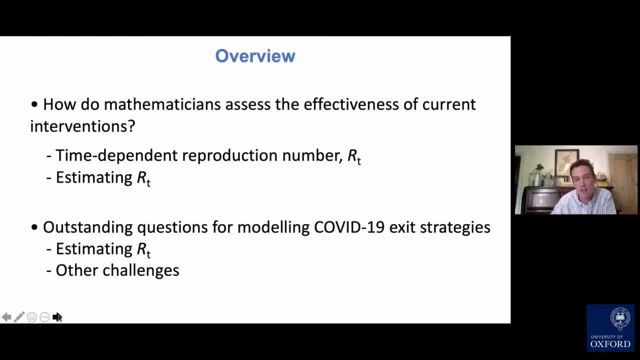 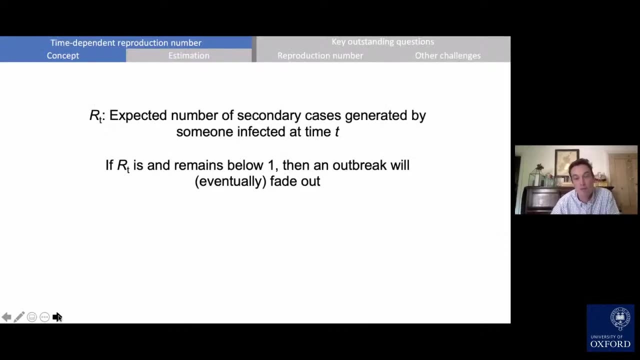 So some of those questions relate to challenges in terms of estimating the R number, But then I'm going to talk briefly about other challenges for predicting the effects of different possible exit strategies from this pandemic. So the time dependent reproduction number, the R number or RT, that's the expected number of secondary cases generated by someone who's infected at time T. 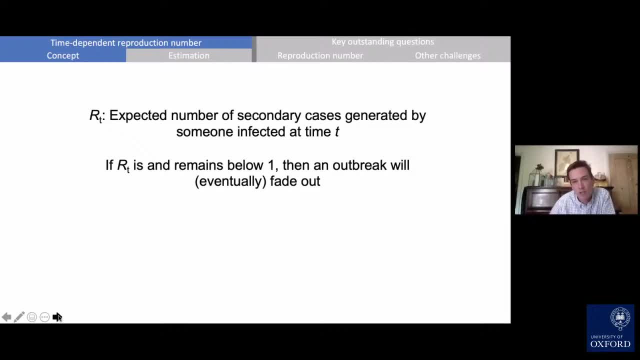 And so if RT is below one and if it remains below one, well, that means that the epidemic is eventually going to fade out, right, That means that each individual, on average, is infecting less than one person, And so, gradually, case numbers are likely to decline and fade out. 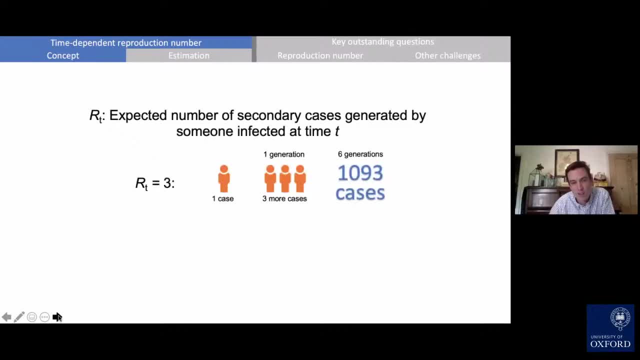 If instead the R number is bigger than one, though, then the R number is going to fade out, So that means that each individual on average is infecting less than one person. So if we're in a situation in which the time dependent reproduction number is three- and let's say that it remains at three going forwards- then the picture is very different. 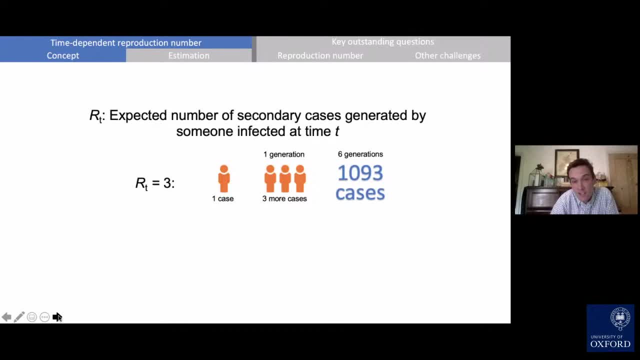 And the picture in that case is that you have one initial case starting a chain of transmission. On average, that one initial case is going to go on and infect three individuals in total. So in the first generation of infection you've got three more cases in addition to your first case. 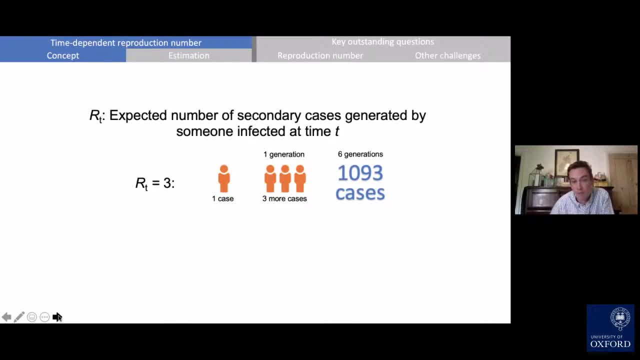 And each of those three infected individuals- if the reproduction number remains at three- will go on and infect three more individuals. So in the second generation of infection you've got nine cases in total, And each of those nine will go and infect three more individuals. 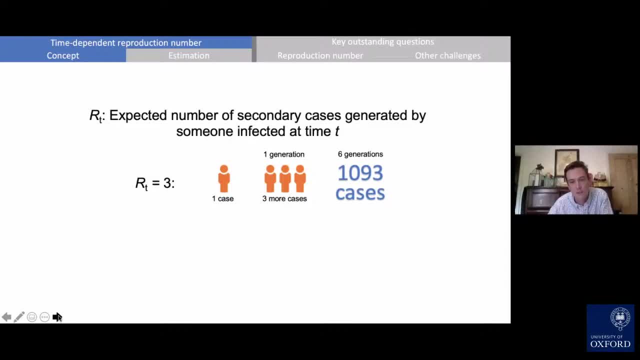 So in the third generation you've got 27 cases and so on, And that's going to continue if the reproduction number remains at three, So that after six generations in total, cumulatively over all the previous generations, you've got over a thousand cases. 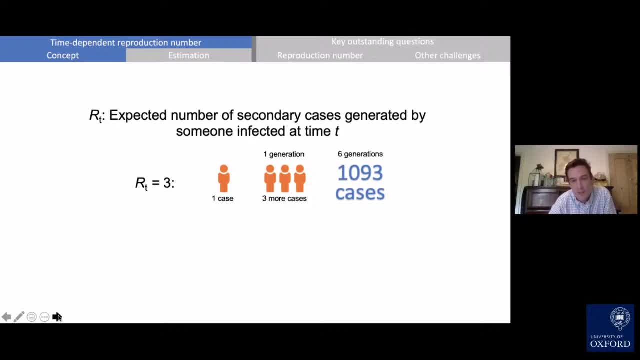 So that's what happens if the R number is and remains at three, But if you introduce public health measures that can reduce the R number. So, for example, let's say that we introduce a public health measure that reduces the contacts that we all have by a third. 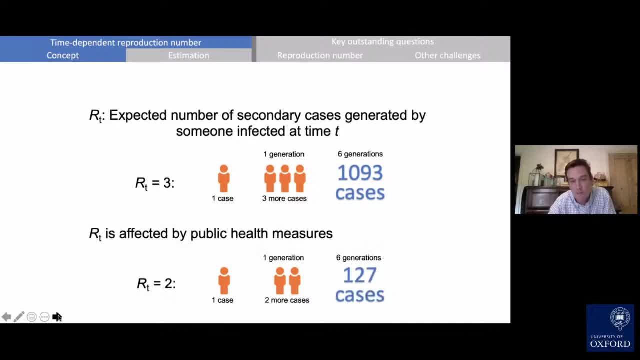 Well, in that case then the reproduction number would fall, and it would be two, because contacts have been reduced by a third. And so now we get a slightly different picture, And this new picture is that your first case, your index case, will go on and infect only two people this time. 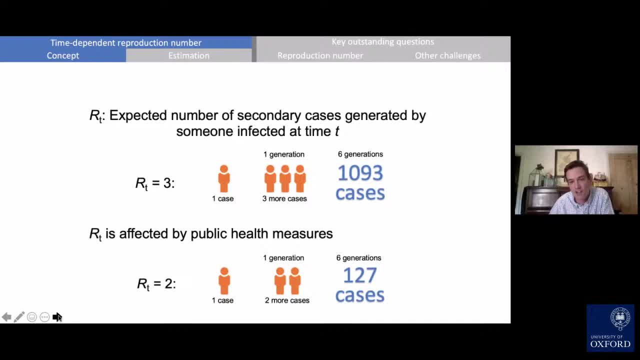 Those two will go on and infect two people each. The second generation will now have four. Those four will go on and infect two cases each. So the third generation of infections will have three cases for each of those four cases, In other words 12 cases, and so on. 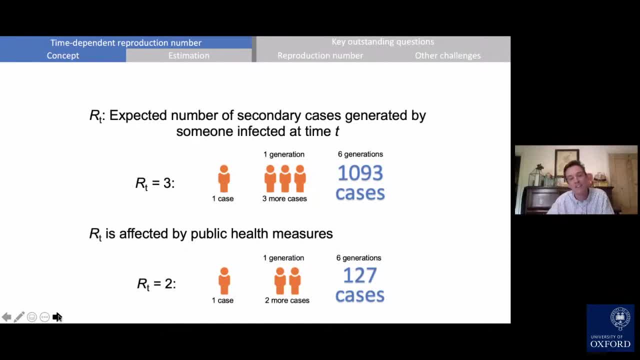 Sorry, two cases for each of those four cases, So in other words eight cases and so on, To the point that after six generations, So now, instead of having over a thousand cases, you instead have just over a hundred cases. And so this shows that if the reproduction number is varied by public health measures, 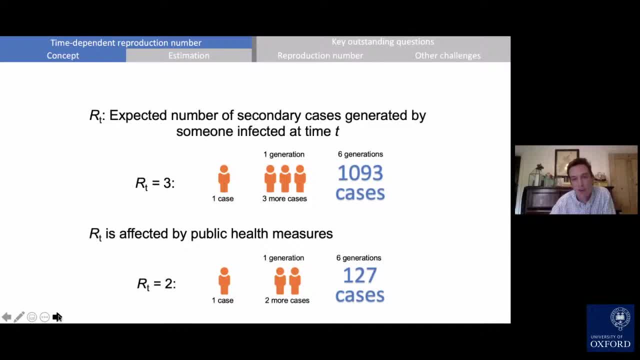 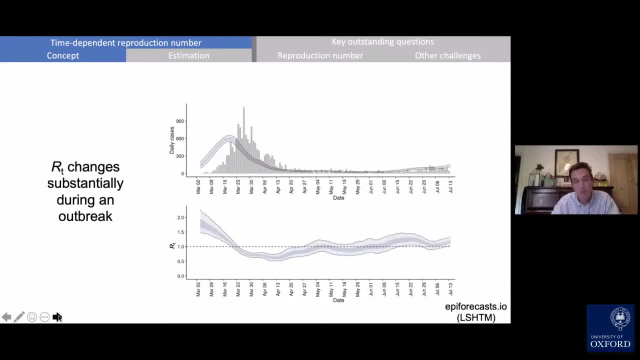 then that will kind of follow through in the number of cases That you observe. So in reality in the two examples I've just shown, I assume that the reproduction number remained at a constant level. But in reality, as an outbreak goes on, the time, dependent reproduction number, or RT, is going to change substantially, and it changes for different reasons. 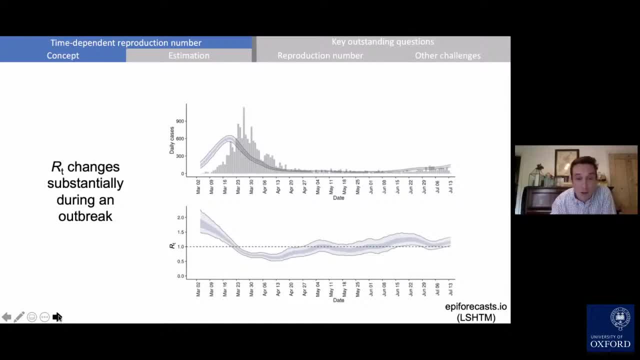 One reason that it might change is that public health measures change, and that's going to affect the reproduction number. Another thing that might change is human behaviour might change in response to the epidemic, And again that's going to affect The reproduction number. 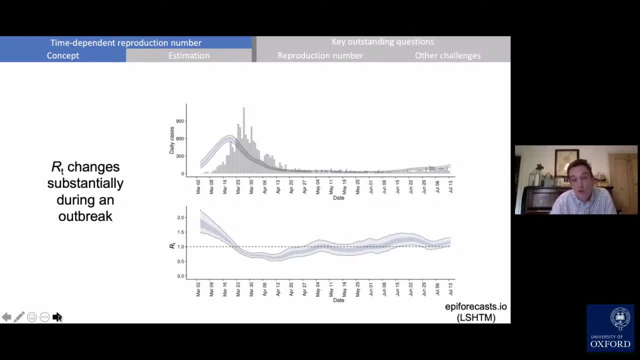 And there are other factors at play too. So, for example, the level of acquired immunity in the population is also going to affect the time dependent reproduction number, And so what you typically see in outbreaks is instead something that looks like the graph on the bottom right. 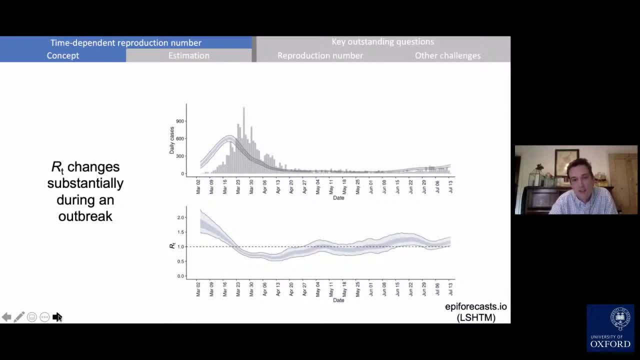 So a reproduction number that actually changes as the outbreak is ongoing. So this is a reproduction number estimate constructed by the team at the London School of Hygiene and Tropical Medicine, And it's based on the grey bars. And it's based on the grey bars. 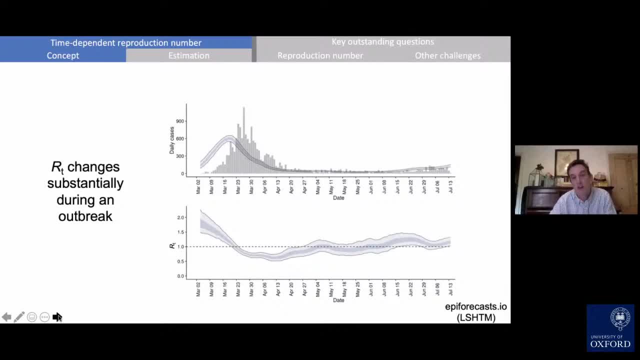 In the top figure. So the grey bars in the top figure are the numbers of reported cases per day of COVID-19 in, I think, Austria in this particular example, And what you can see is that early on case numbers start to go up. 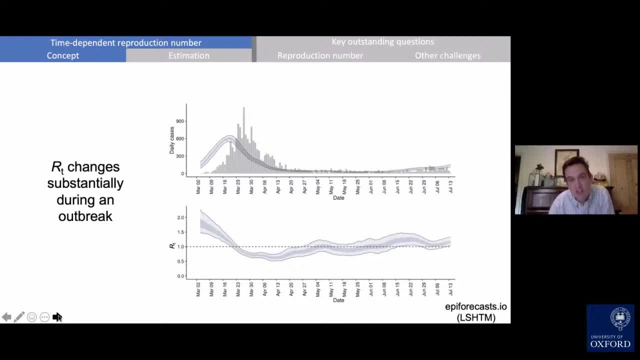 And because case numbers start to go up in the grey bars in the top figure. that means that the reproduction number is bigger than one. cases are increasing, But the rate at which cases are increasing is something that's slowing down slightly. So, in other words, the reproduction number is something that's falling. 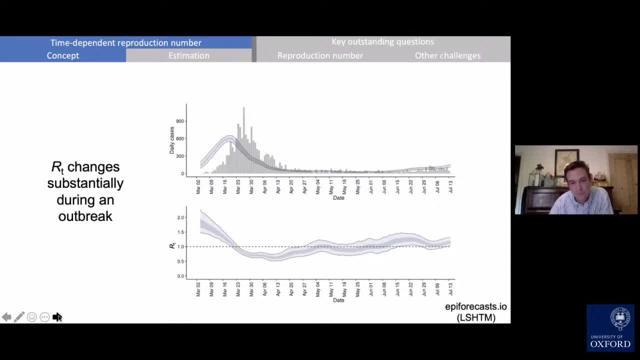 And that's what you can see initially in the bottom figure too. Eventually, what happens is the reproduction number dips down below one, And so case numbers then end up peaking and then coming back down again because the reproduction number is below one. 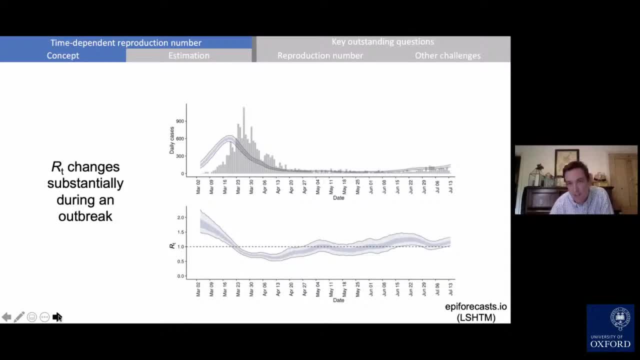 And eventually case numbers sort of stabilise at a very low level. You can see from sort of the end of April up until kind of mid-July in this particular figure you can see that case numbers are pretty much constant. They're at a pretty much constant level. 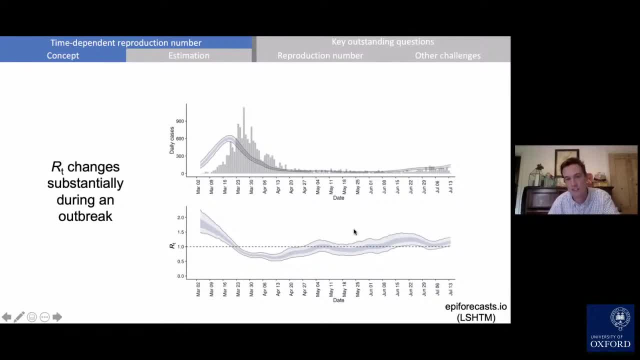 So that means that the reproduction number is approximately one, And indeed you can see that on the bottom figure here that the reproduction number is approximately one in that period. So that means that each individual is infecting, each infected individual is infecting on average one other person. 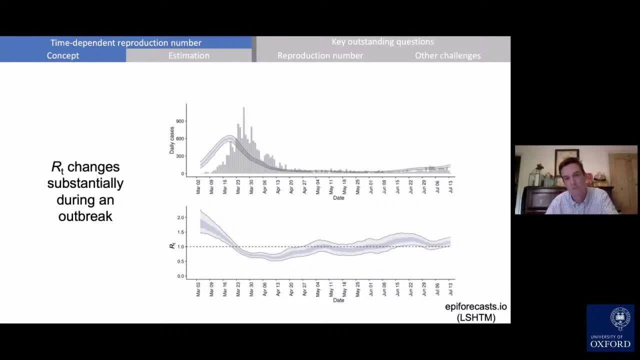 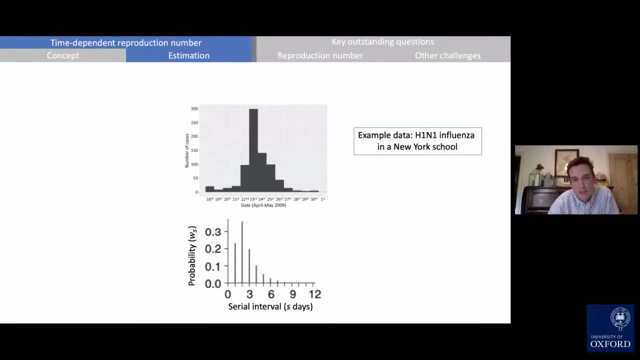 So the case numbers are remaining approximately constant. So that's what it kind of looks like during a real infectious disease epidemic. That's what reproduction number estimates look like. What I want to do now, though. we've heard a lot about the reproduction number in the media. 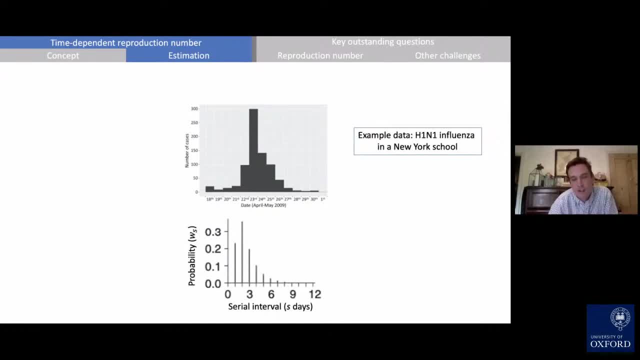 But what I want to do now is I want to look at the number of cases. What I want to do now is I want to show you how the reproduction number, more precisely, is estimated, And so the method that I've been using to do this involves two types of data. 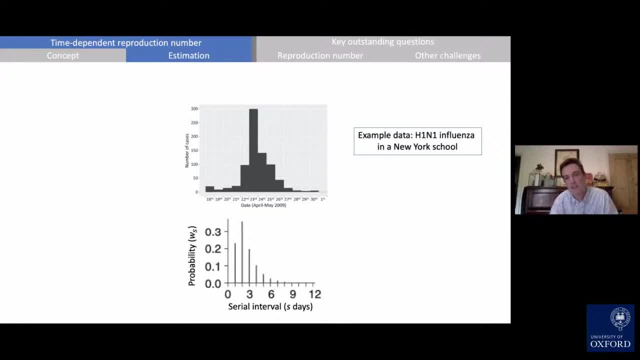 The first type of data is data on the numbers of cases per day. So this is an example. This is from from the H1N1 influenza pandemic And this is numbers of cases per day in a New York school, And then what you've got in the bottom figure is the other type of data that you need in the bottom figure. 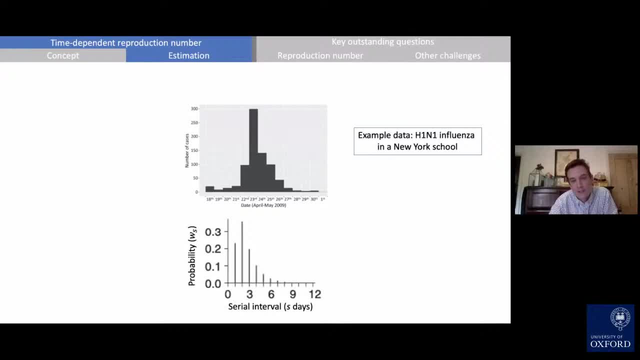 What you've got is you've got an estimate of the number of cases per day And then you've got a serial interval. So that's the other kind of data set that you need, And the serial interval describes the time between successive cases in a chain of transmission. 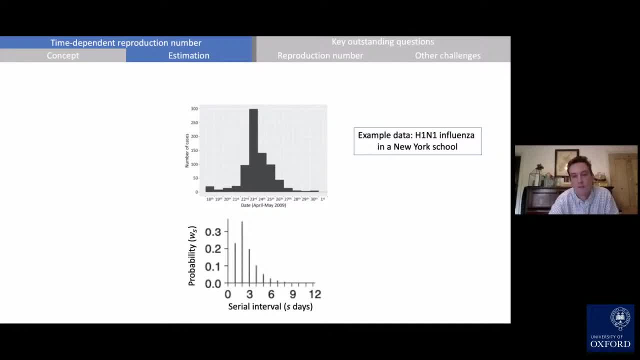 So what it describes is: so suppose that I end up contracting a particular disease and I show symptoms on a certain day, What the serial interval says is: it says: when will individuals that I go on to infect show symptoms? So in particular, looking at this exact figure here, what this exact figure here is saying is that if I go and infect someone else, 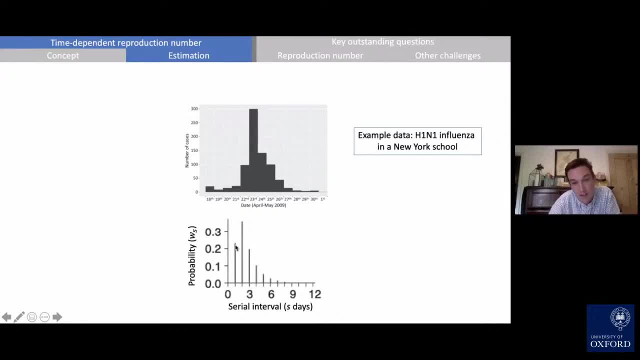 there's about a 23 percent chance that the person that I infect show symptoms the day after me. There's about a 35 percent chance the person that I infect show symptoms two days later. There's about 20 percent chance the person that I infect show symptoms three days later, and so on. 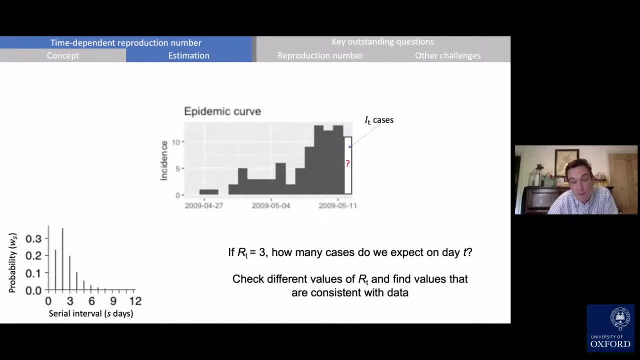 So the question then is: how do we go about estimating the time dependent reproduction number in real time during the outbreak? Well, what you do, if you want to estimate the reproduction number, if you want to estimate the reproduction number on day T, what you do is the following: 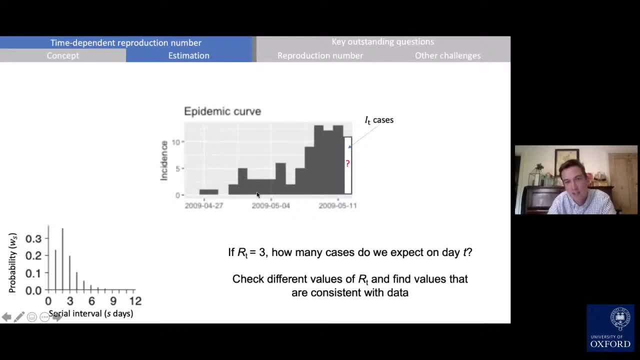 You look back at the numbers of cases that have been seen in all days before day T, And then one way that you can estimate the reproduction number is simply to take a guess as to what the reproduction number is in the first instance. So you might guess, for example, that the reproduction number was three. 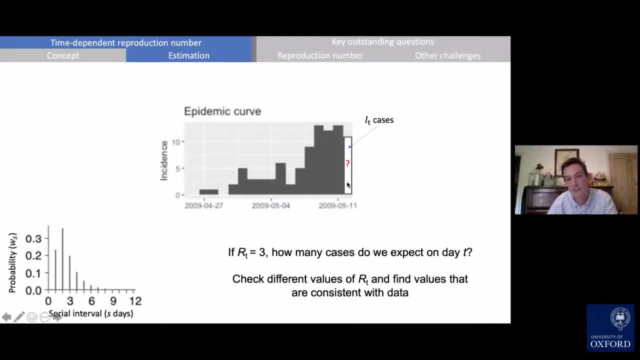 Well, if the reproduction number was three, you can calculate the number of cases that you might expect to happen on day T. And the way you do that is: you say, well, on day T minus one there was some number of cases. 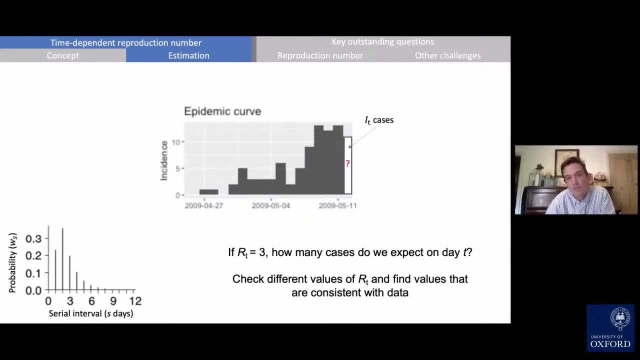 If the reproduction number was three, then each of those cases will go on and infect three individuals each, And the number of those kind of onward transmissions that you'll see in the data on day T, the proportion, corresponds to the probability that the serial interval is one day, because you need the cases on day T minus one to generate cases one day later. 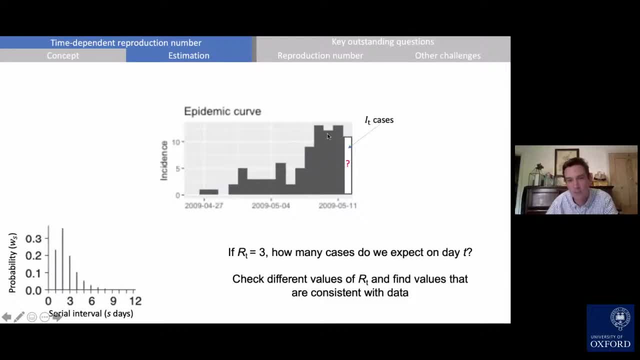 Then what you do is you look back earlier in the application, Earlier in the epidemic. So you would say, let's look at day T minus two. Well, all of the cases on day T minus two will generate three cases each, And the proportion of those three cases that appear on day T according to the serial interval is about 35 percent. 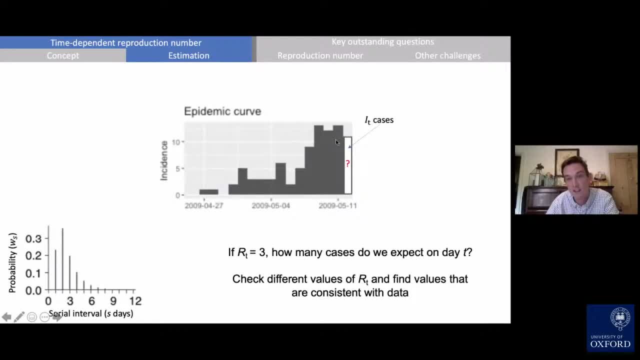 And so that gives you an estimate for the number of cases on day T coming from individuals that appeared as cases on day T minus two. And then you can go back to the previous day and you can say: well, on day T minus three, there was some number of cases. 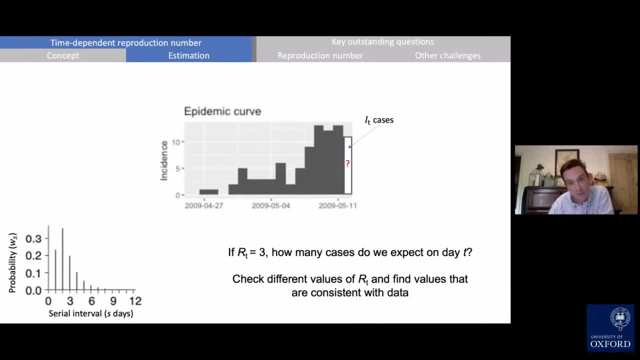 Each of those will infect three Individuals each if the reproduction number is three, And the proportion of those that will appear on day T corresponds to this proportion here, ie about 20 percent, And so by summing over all previous days you can then construct an estimate for how many cases you expect to see on day T if the reproduction number was three. 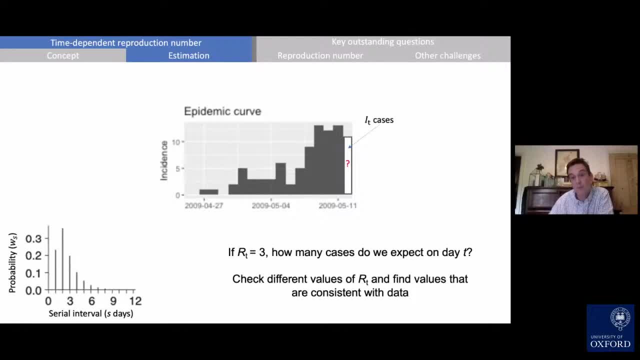 So what you can then do is you can actually look at how many cases really appeared in the data on day T And you can compare that to the number you predicted if the reproduction number was three. And so if the number of cases that actually happened was larger than the number that you predicted, if the reproduction number was three, then that means that the reproduction number has to be larger than three. 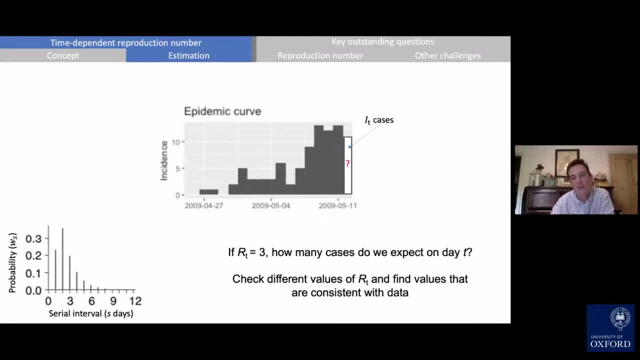 If the number of cases that actually occurred on day T was smaller than the number that you predicted. if the reproduction number was three, then that means that the reproduction number has to be smaller than three, And so in each case, you would then make another guess for the reproduction number. 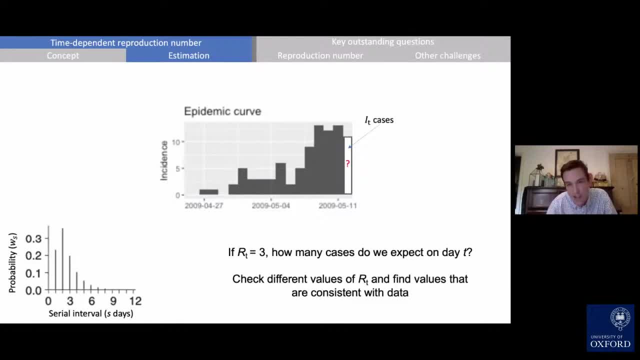 And you could gradually sort of iterate, gradually, sort of iteratively converge in on the right estimate for the reproduction number by adjusting your estimate based on the number that you would expect to see compared to what actually happened. so you can essentially just check different values of the reproduction number. 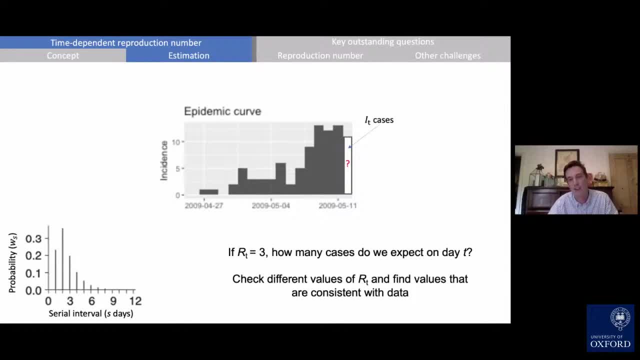 and find the values that are most consistent with the number of cases you actually saw on day t, and so that provides a way to estimate the time dependent reproduction number. there is a slight problem with this issue, with this particular particular method for estimating the reproduction number. there's a slight issue with this, and that slight issue is that it generates 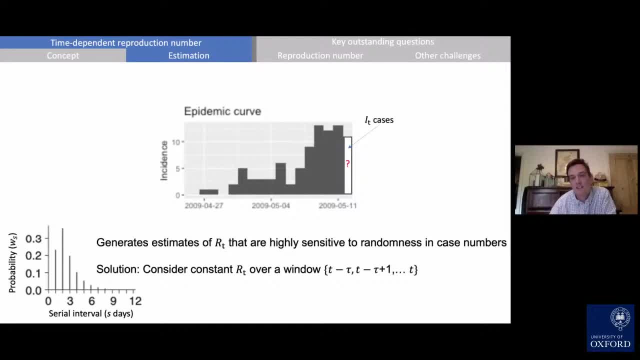 estimates of the time dependent reproduction number that are very sensitive to randomness in case numbers. so, in reality, if the reproduction number had a constant value, there'd still be some randomness in the number of cases you see each day, and so if the number of cases you see each 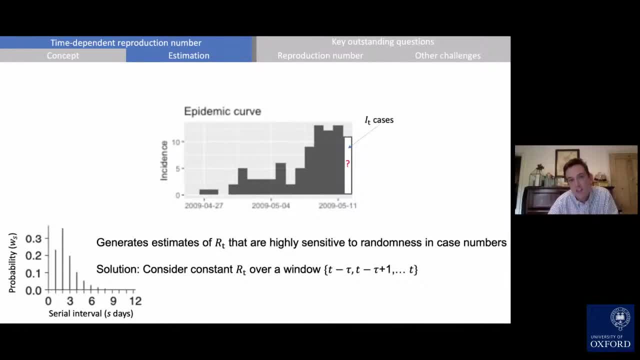 day is something that kind of randomly changes the time, dependent reproduction number then kind of fluctuates slightly, then that will be translated into estimates of the reproduction number, so you'd get estimates of the reproduction number. that also kind of jag around every day. and so to to get rid of that sort of jagging around from day to day, what you do is you say: 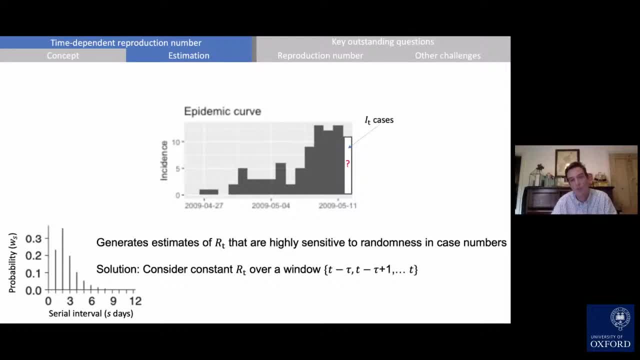 well, let's assume that the reproduction number is constant within some time window. so, for example, you say every five days. we'll assume that there's a constant value of the reproduction number and, rather than using the data from day t to estimate the reproduction number, you use the data from. 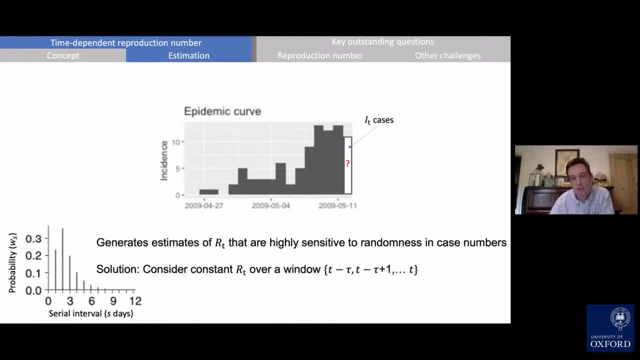 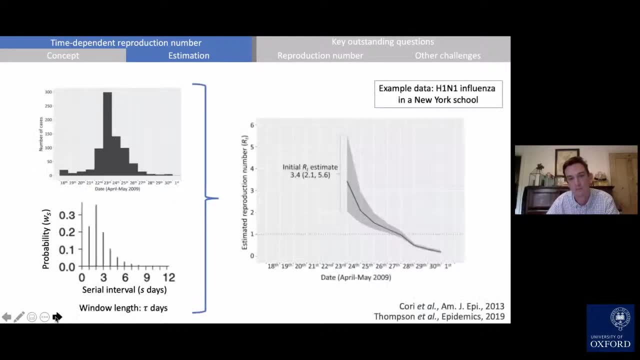 day t and also the four days before that in order to estimate the reproduction number. so you have a window of five days which makes the estimates, the reproduction number, smoother, so the output then. so this is all a bit technical, but the key thing to take away from this is what you get in the end. 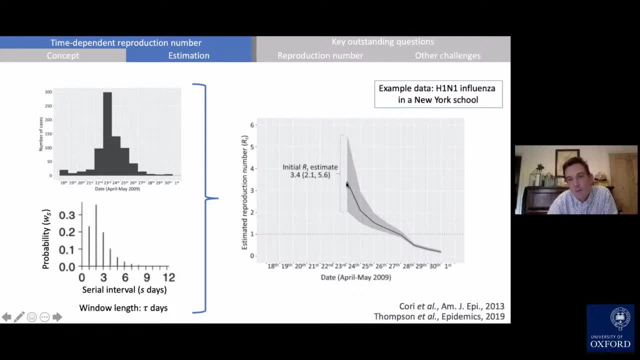 is you get an estimate of the reproduction number that might look a little bit like this, whereby your estimate for the reproduction number on this day depends on the number of cases that day, but also the number of cases on the few days before it. your estimate for the reproduction number on 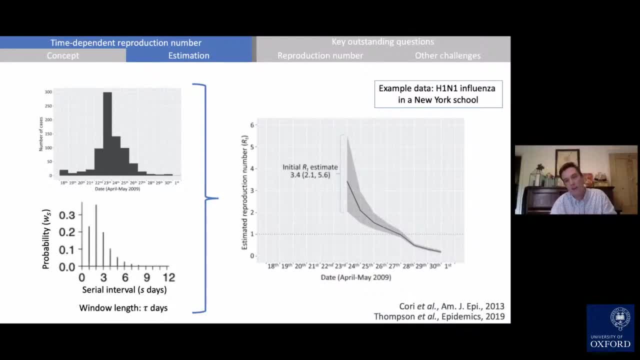 this day depends on the number of cases on this day, but also on the few days before it and so on, and then, by using this approach, you can just track changes in the reproduction number as the outbreak goes on. okay, so that's, that's kind of how we estimate the reproduction number in real time. 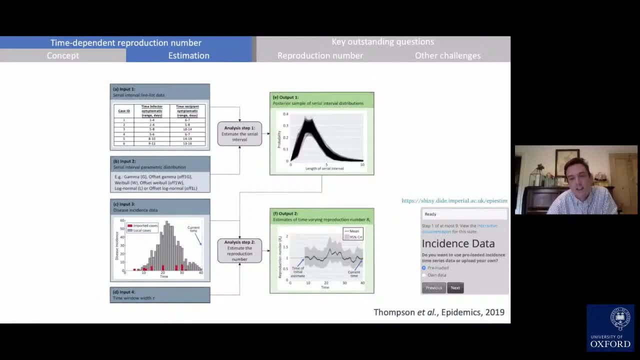 during epidemics and some work that we did last year extended this basic method. the key extension of this method for covid19 is that we also developed a user-friendly software app where you can upload your own data. so there's actually a website, so it's this website here, and on that website you can upload your own data. so data for the numbers of 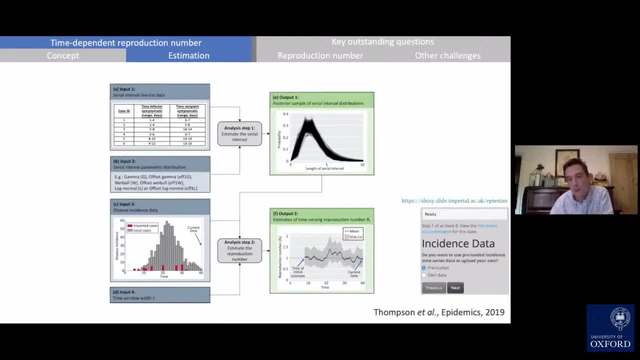 cases per day, and then what the website will then tell you is. it will. it will output an estimate of the time varying reproduction number based on the data that you upload, and this website and this and this tool has been used a large number of times during the covid19 pandemic. 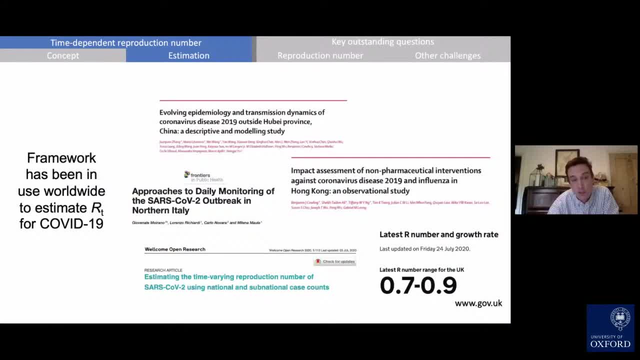 so the framework that i've described so far, as i say, has been used worldwide to estimate the time dependent reproduction number during the pandemic. as i said a little bit earlier, a number of different groups have been estimating the r number throughout the pandemic for the uk, and contributions from all of those different 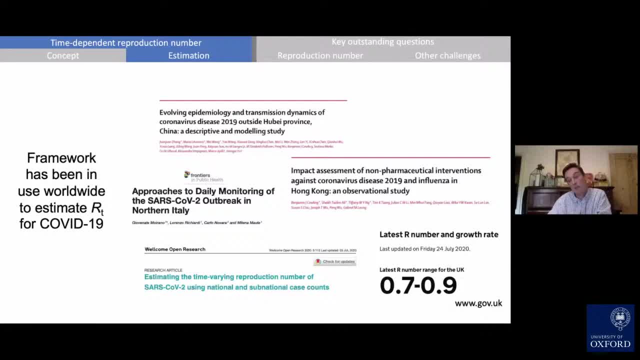 groups are then put together to then come up with a range of kind of plausible r values representing a range of different mathematical models. but a lot of those mathematical models are based on the framework that i just showed to you, so they're all this kind of fairly simple. 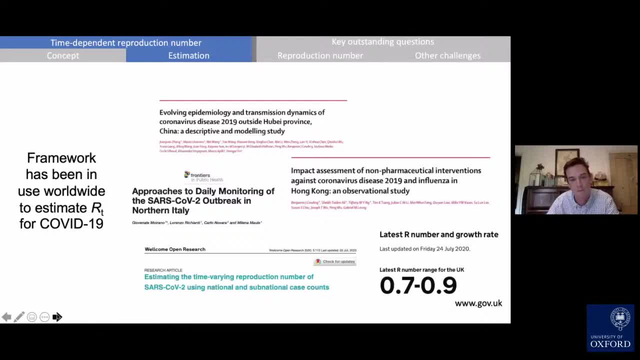 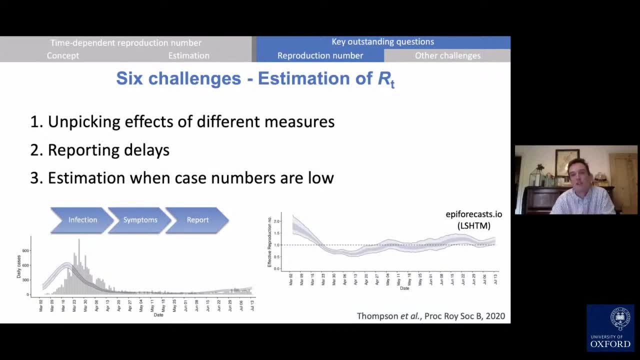 statistical framework for estimating the time-dependent reproduction number during the pandemic. so we're going to talk about some of the most common ways that we can estimate rt. so now i'm just going to talk about some outstanding kind of challenges, firstly for estimating rt, but then more generally for predicting the effects of different possible 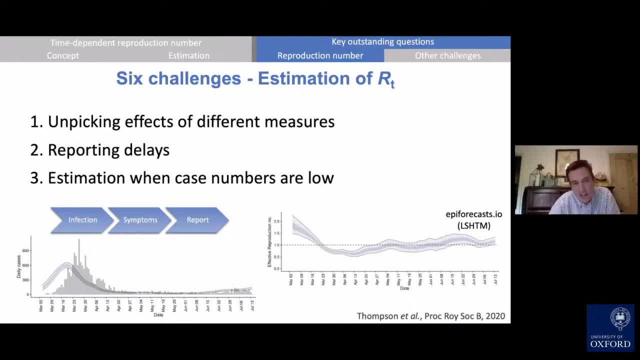 covid19 exit strategies. one of the key challenges at the moment is to be able to unpick the effects of different control measures. so if we see the reproduction reproduction number dropping, what that tells us is that control measures are having a very positive effect, but it doesn't necessarily tell us if lots of interventions are introduced all at the same time. 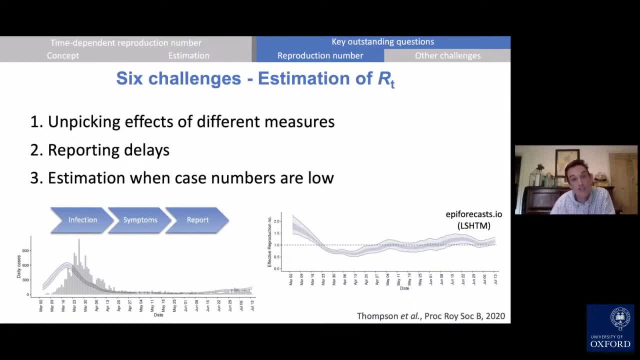 which one of those interventions are having the largest effect and, therefore, which intervention is most important. so, going forwards something that's very important: it's going to be unpicking the effects of different control measures, understanding the different aspects of the lockdown that led to a fall in the reproduction number, something else that's. 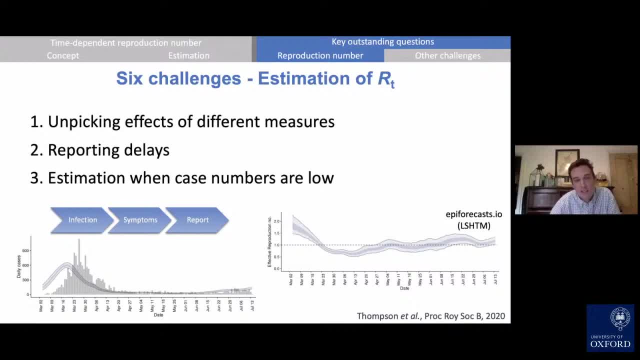 had a lot of attention recently is reporting delays. so, typically, in the method that i just described, what you do is you take data on the numbers of cases that's being reported and what's, And you use that to estimate the reproduction number. What you really care about, though, is you care about disease transmission. 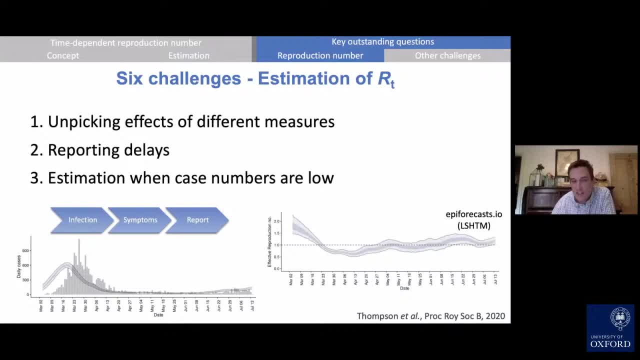 So, in other words, you care about the number of infections that are happening, And the data that we have is not the number of infections that are happening, but it's data on the numbers of reported cases. When someone's infected, there's then a delay before that person shows symptoms. 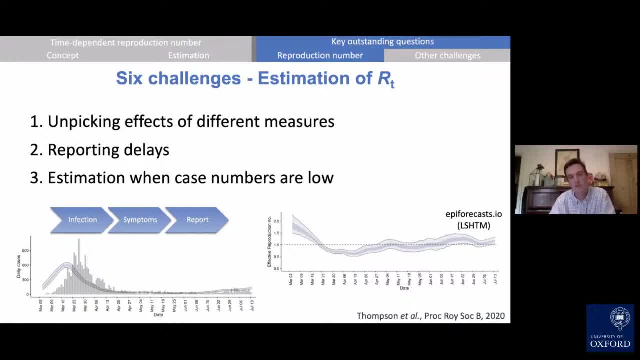 It's called the incubation period. Right, They get infected, There's a delay before they show symptoms. There's then a further delay before they then report their infection, And so the data that we get for for reported cases is not the same as the data on the number of cases that have occurred. 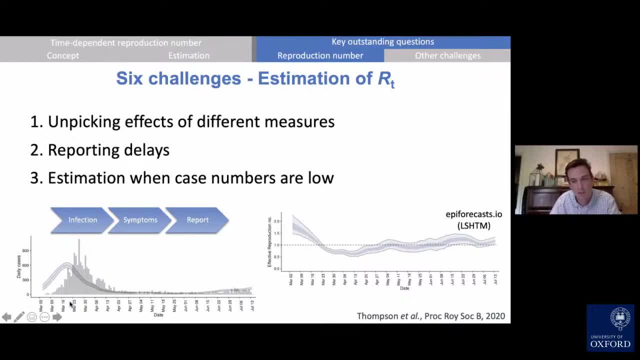 And there are methods that have been developed for handling this. So here's one example that's being used by the London School of Hygiene and Tropical Medicine. The grey bars are the reported cases. What they do is they then sort of back calculate from the reported cases the numbers of infections per day. 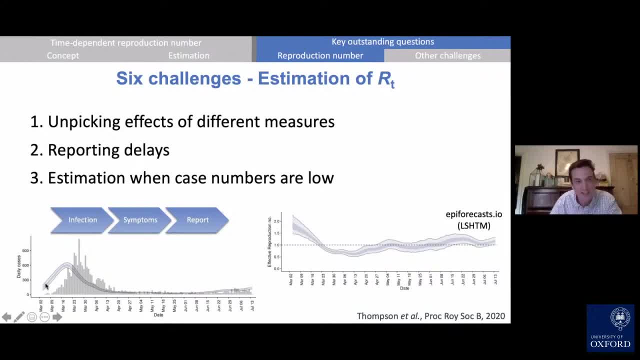 So that's what's given by the shaded area here. This is an estimate for the number of infections per day, Based on the numbers of reported cases, And then what they do is they estimate the reproduction number using data or using these kind of estimated number of infections per day, rather than using data on reported cases. 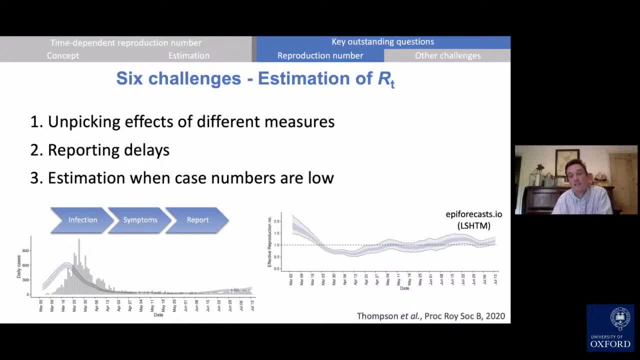 Something else that's likely to be very important going forwards is to come up with ways to estimate the reproduction number when case numbers are low. So typically, when case numbers are very low, there's very little data with which to estimate the reproduction number, And so reproduction number estimates tend not to be very important. 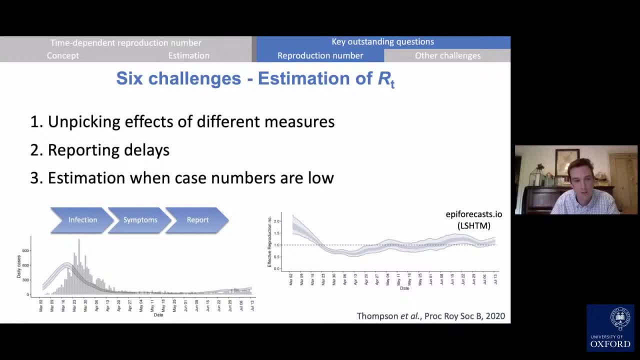 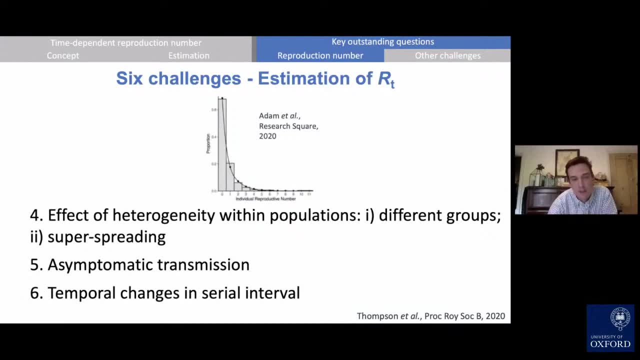 They tend not to be as accurate, And so that's something that it would be good to address going forwards. A few more challenges when it comes to estimating RT. I'll just talk about one of these. So, in particular, I'll talk about the top one. 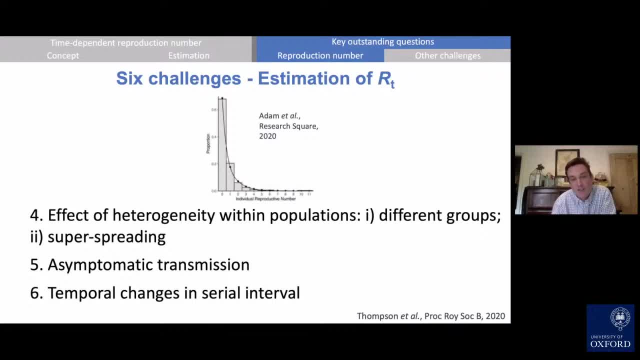 So something that's very important in terms of the reproduction number is the effects of heterogeneity within populations, and indeed between populations too. In particular, different groups transmit any infectious disease or any pathogen very differently, And so the value of the reproduction number might be very different in different groups. 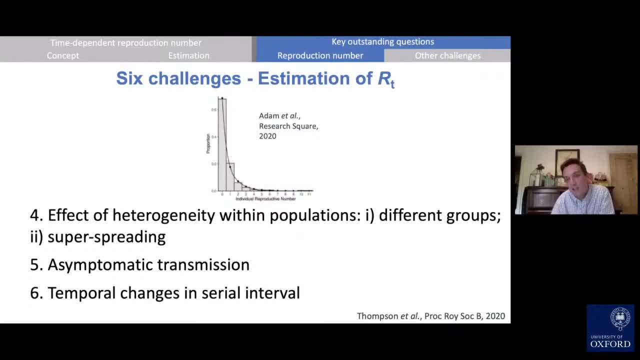 So what it would be very good to do is actually to have data on transmission in different groups. You might have data, for example, on transmissions within care homes compared to within the rest of the community, And if you have that data then you'd be able to estimate reproduction numbers differently in those different groups. 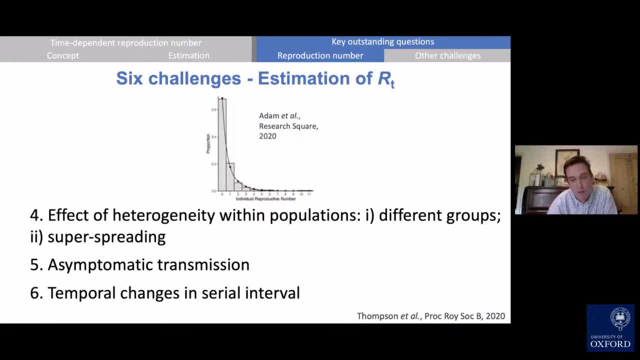 I think understanding heterogeneity between different groups is something that's likely to be very important going forwards, And then a related thing is the idea of super spreading. So there's a general rule of thumb for pathogens, kind of generally, which is that around 20% of infected hosts tend to contribute about 80% of transmissions. 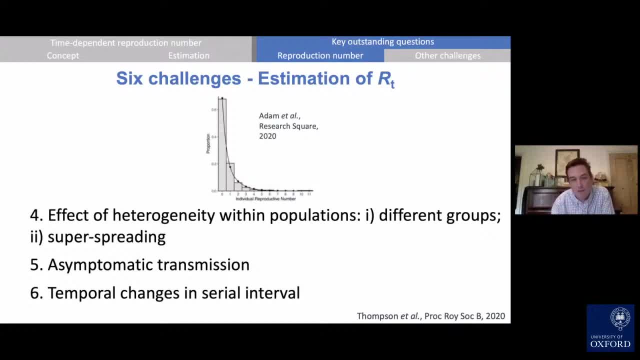 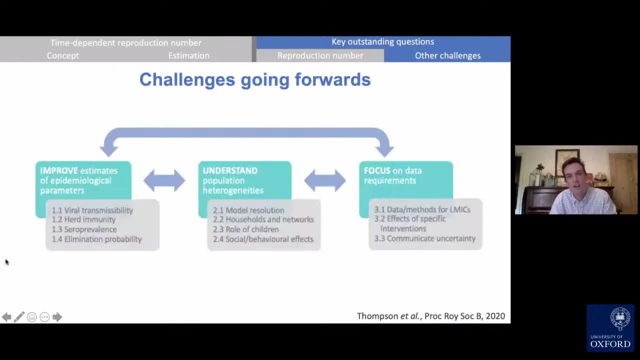 And so it's not the case that everyone in the population has a reproduction number of three, but actually there's a substantial variation between individuals, And that variation between individuals is something which is a focus of current research efforts. So then, finally, then, I just wanted to highlight some challenges going forwards if we want to make predictions using mathematical models. 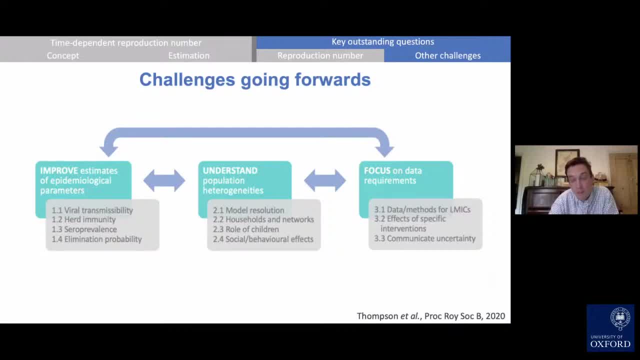 So I'm going to start off by talking about the effects of different exit strategies. I've just written a paper with a few few other mathematical modelers from around the world, many of whom are advising governments, And that paper is called Key Challenges for Modelling- COVID-19 Exit Strategies. 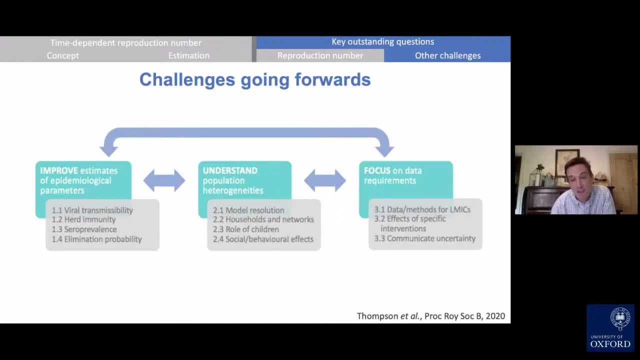 And it's about to be published in Proceedings of the Royal Society B And there's a preprint of that manuscript that's available online. And what we do in that manuscript is we outline a number of different key challenges that are mathematical modelling, predictions of the effects of different exit strategies. 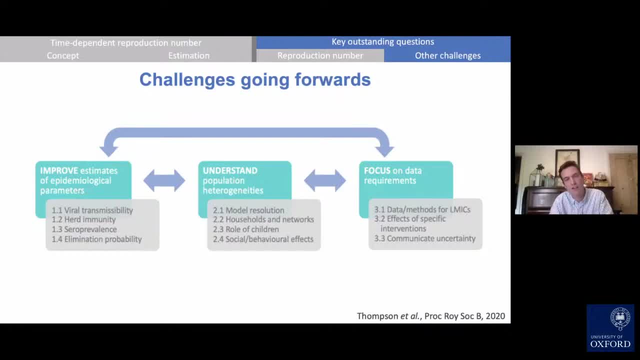 And broadly the challenges fall into three different groups. The first set of challenges are about estimating epidemiological parameters more accurately, So that includes parameters like the time dependent reproduction number. The second thing that I think you know, the second area that's going to be very important going forwards- is understanding population heterogeneities more clearly. 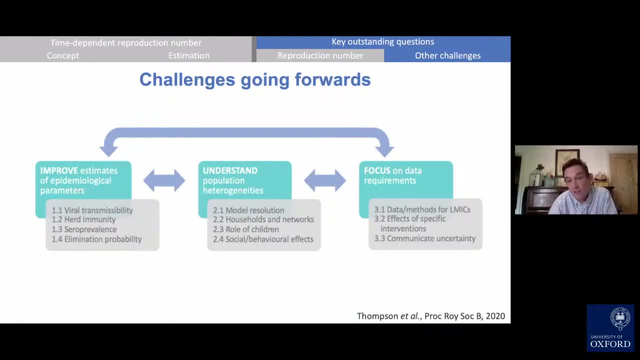 So, for example, understanding more clearly the role of children in transmission compared to adults. That's going to be very important in terms of strategies regarding when to open schools and workplaces. And then, finally, the other thing that needs to happen is there needs to be a focus on data requirements. 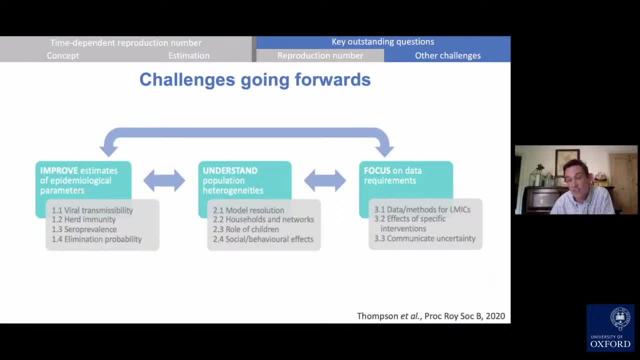 So there needs to be a concerted efforts to identify the precise data sets that need to be collected in order to be able to predict the effects of different exit strategies more precisely. So, with that, I'm going to leave it there. I'm just going to conclude by saying that the time dependent reproduction number. 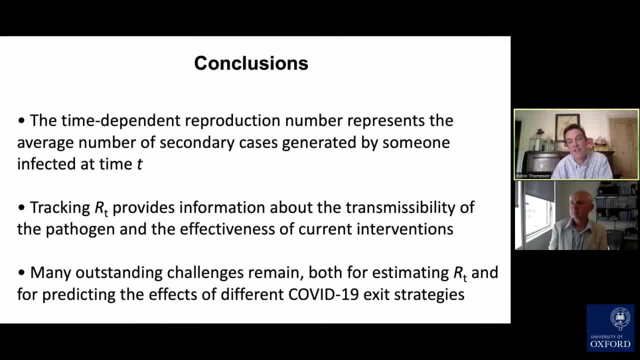 or the R number or RT, represents the average number of secondary cases generated by someone that's infected at time T. If you track the value of the time dependent reproduction number, that can provide information about the transmissibility of the pathogen. in the case of COVID-19,, the virus 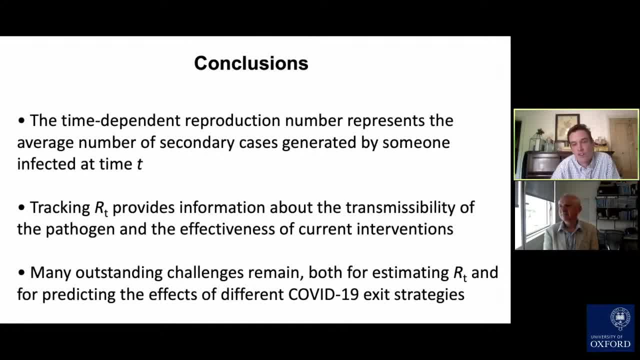 And it can tell you how effective current interventions are. So if RT is less than one, then current interventions are doing a pretty good job, Whereas if RT is greater than one, then you would expect case numbers to increase too. And finally, I talked about how many. 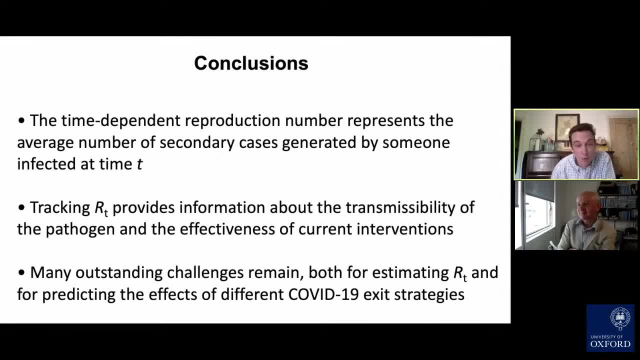 how many outstanding challenges remain there for estimating RT, but also not only for that, but for predicting the effects of different COVID-19 exit strategies going forwards, And so with that I think there's some time for questions. I'm going to hand back over to William now And thanks very much for tuning into this COVID conversation. 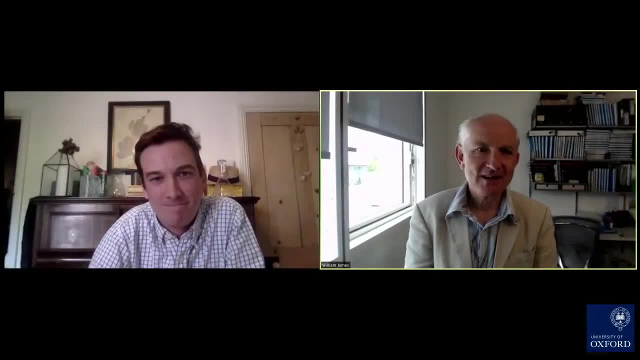 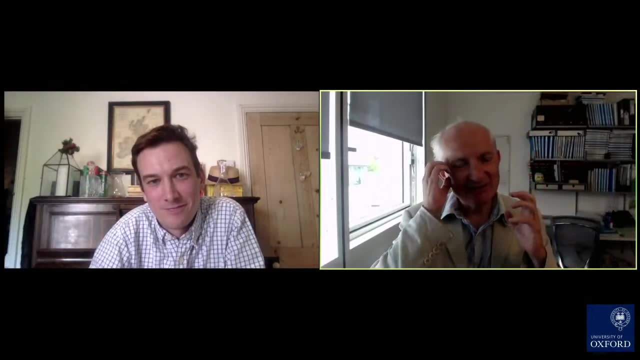 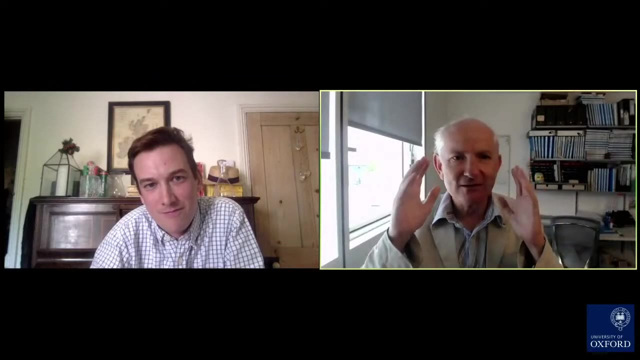 Thank you very much, Robin. That was a really fascinating talk, And the sign of a really good talk from my point of view is there's something that I've not understood and haven't really been able to even think through on my own, And when you were explaining how RT can be calculated, it all seemed so very, very obvious and intuitive. 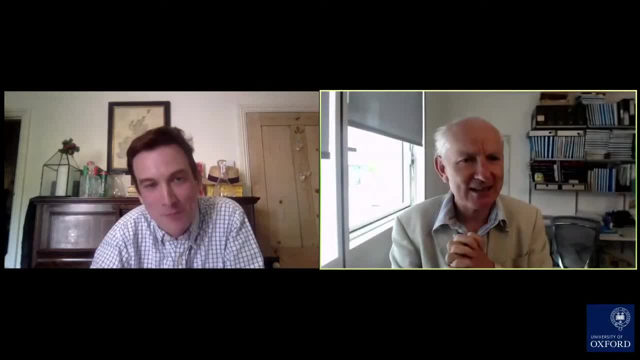 And you convinced yourself you could do that calculation if you just sat down for long enough. That's a great achievement, And you've really brought it to a level that we can, I think, all appreciate. You stimulated the audience, I have to say. There's lots of really good questions there. 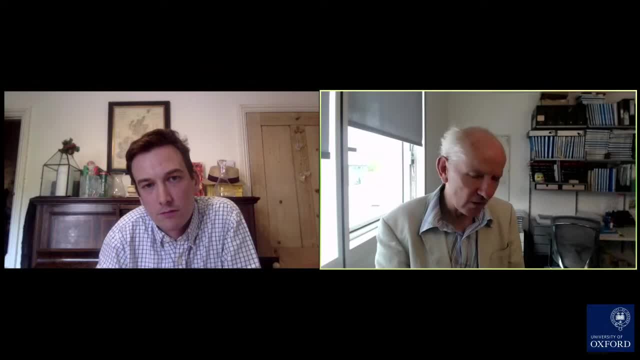 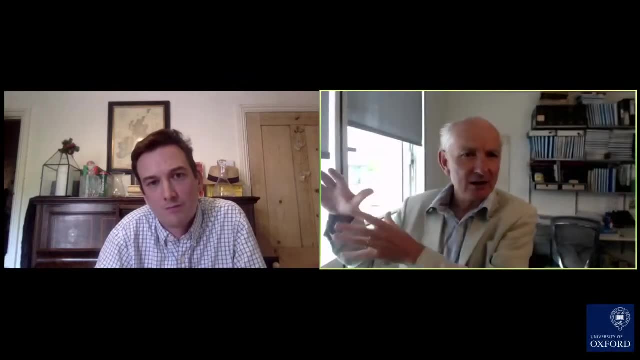 And I think we, What I'm going to do is try and group them, and I'm going to start with the ones that are nearest to the science-y sort of thing and gradually get into policy and then culture and that sort of thing, because it seems like a logical progression, if I may. 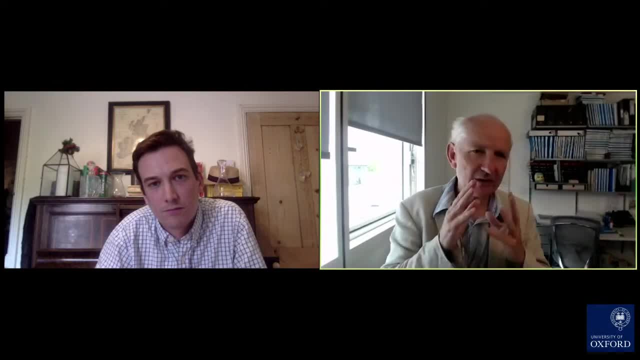 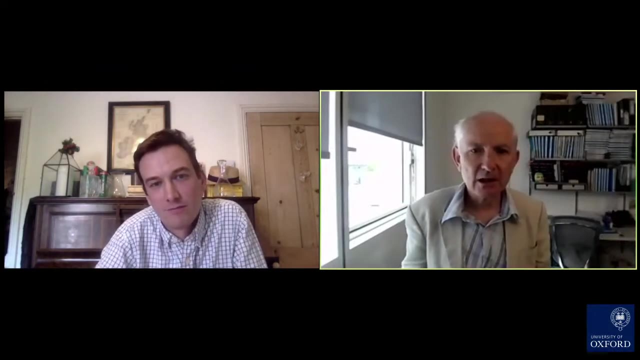 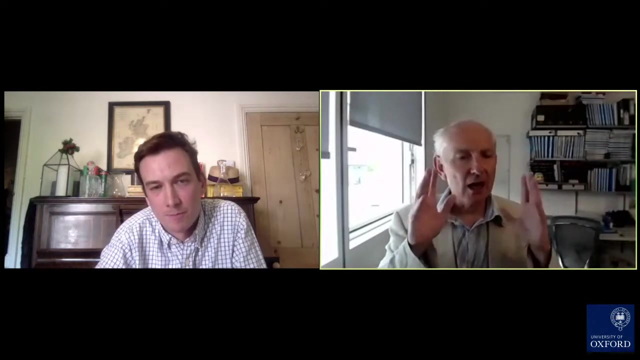 So the two things that were occurring to me- and a couple of our listeners have brought them up- is Very nice. Charlie has brought up one that I was concerned about is that the serial interval graph, the distribution of serial intervals. 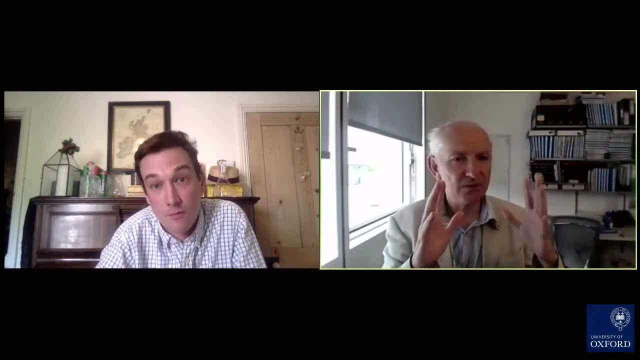 is taken, I think, as a fixed property of this virus. You were showing us the flu one. Yes, that's right, And you need to use that graph in order to do the calculations. Is it actually itself fixed or does it change? 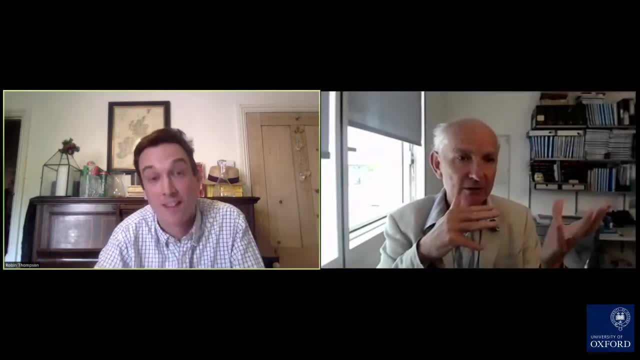 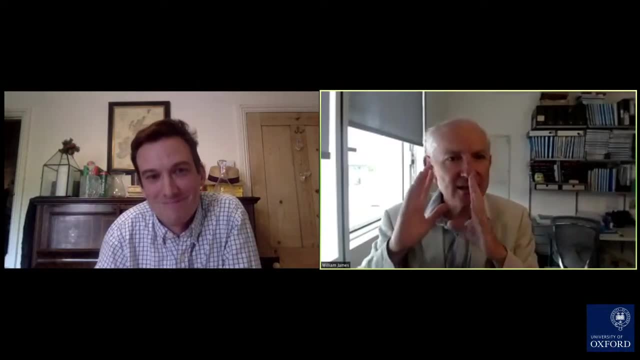 And of course, you don't know it at first, do you Right? yeah, yeah. And does it change? And Charlie's point is: does it itself? I can't think my way through this, you can help us. Does it itself change in response to interventions? So yes, it absolutely does. That's a really great question. So if imagine, for example, that you have a control strategy that involves isolating symptomatic hosts, typically that's going to happen, perhaps after someone's been infectious for a certain period. 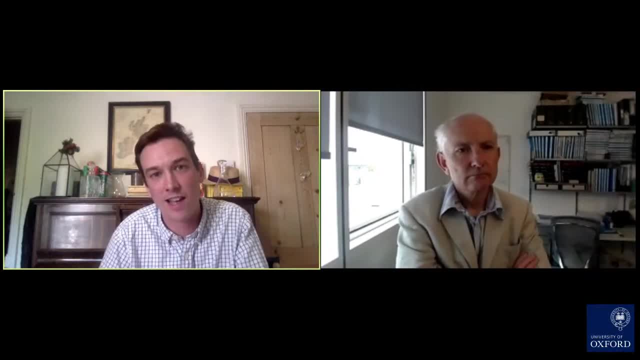 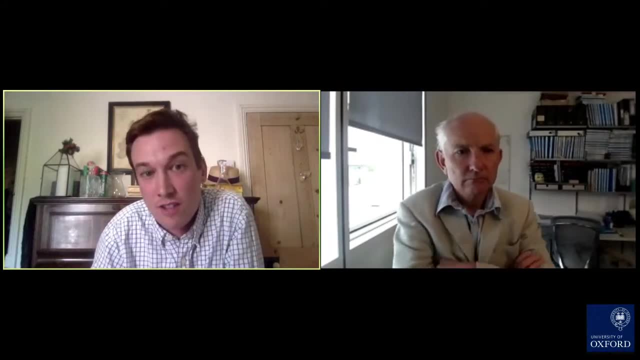 That means that longer serial intervals are perhaps less likely to happen because they're more likely to transmit early an infection. So Charlie's actually right. It's absolutely true that the serial interval is going to change as an epidemic goes on. I think that's a very important target for current research, because most of the serial intervals that are being used in current literature 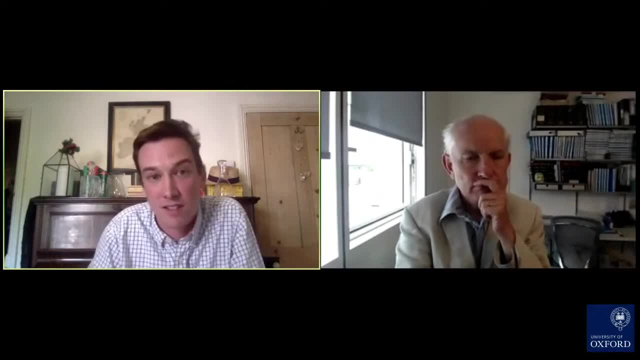 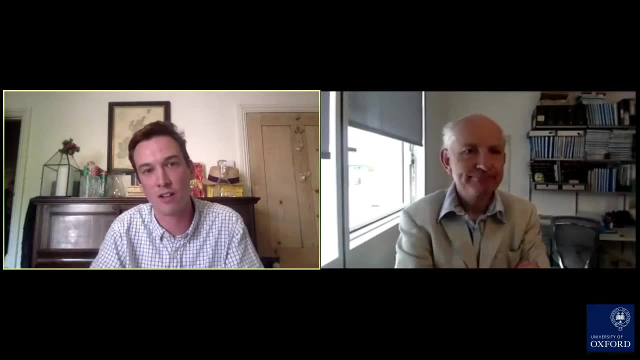 are serial intervals from right back at the beginning of the outbreak. There are estimates that came from household studies where you've got infector and infectee pairs, you've got people that you know infected each other. You look at those individuals and you estimate the serial interval. 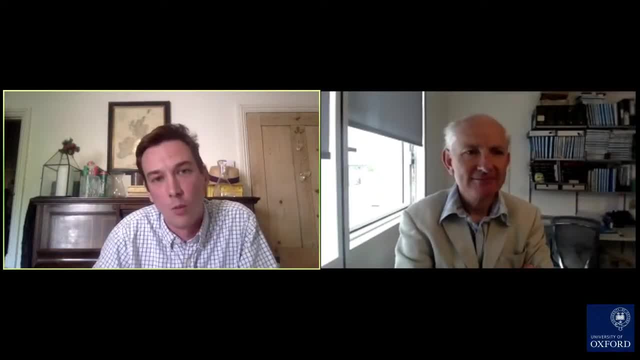 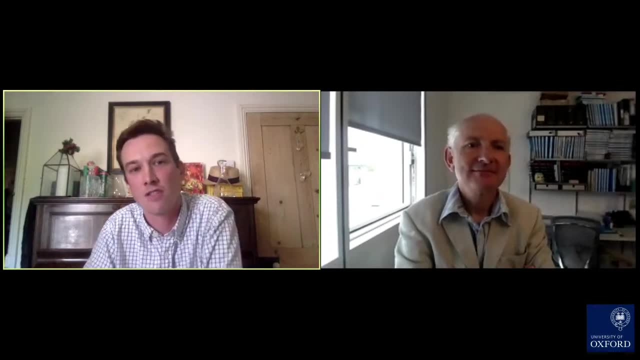 Something that will be an absolutely fantastic bit of research now would be to kind of update that by doing household studies now, not only later in the epidemic but also in other locations. So yeah, absolutely On board cruise ships as well, I think, wasn't it? 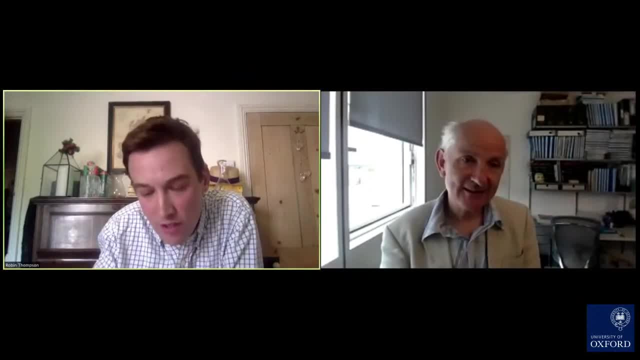 Yeah, exactly, exactly, exactly. And yeah, I think all of those estimates need updating now and that should definitely be a target for current research. There is something, if I may. There's a kind of quite interesting point about serial intervals for COVID-19,. 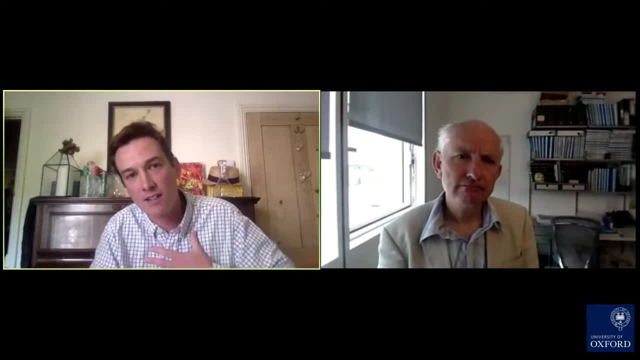 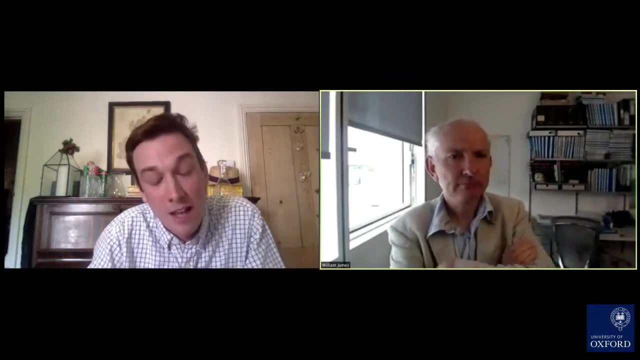 which is that in principle, the serial interval is: if I develop symptoms and then someone else does, it tells us about that interval between symptoms. Yeah, But for COVID-19, there's actually a chance that people can infect other individuals before they develop symptoms. 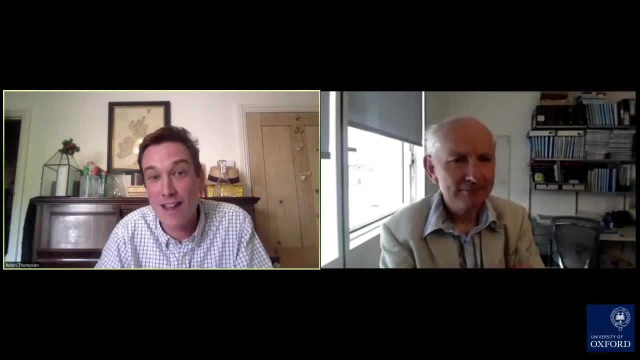 About a 40% chance, I think. isn't it About 40% exactly, indeed? And so that raises quite an interesting point, which is that, actually, if you get negative serial intervals, whereby I might infect you but then you might show symptoms first, 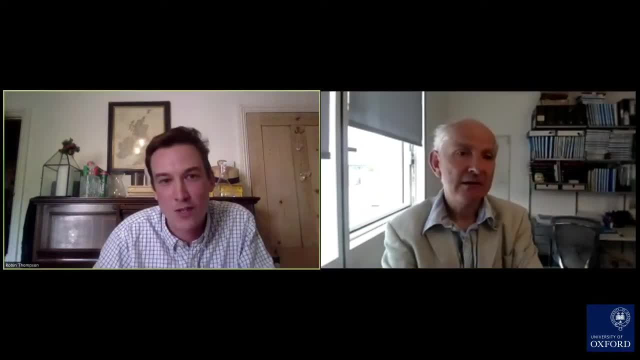 And I didn't have it. yes, So, yeah, so that's kind of an interesting, kind of curious thing, and something again that is quite challenging to model and include in methods for estimating reproduction numbers, But that's not included at the moment in the 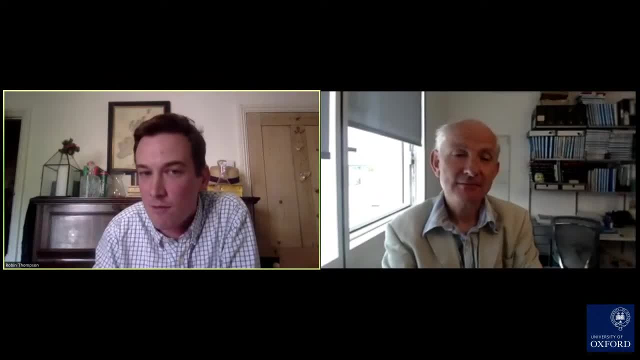 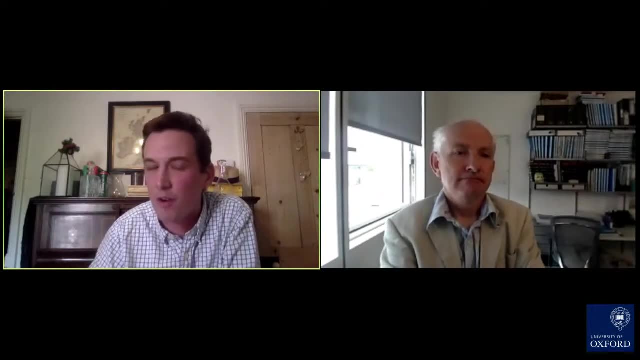 So in the method I just described, pre-symptomatic infection can be there Right, But negative serial intervals are not included in the method that I just described. There are other approaches that can be used and adaptations of this approach that can exist. 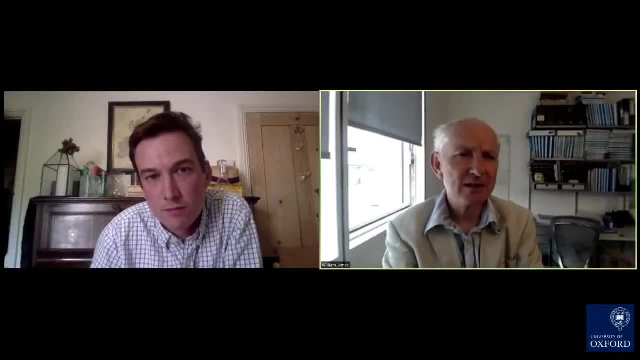 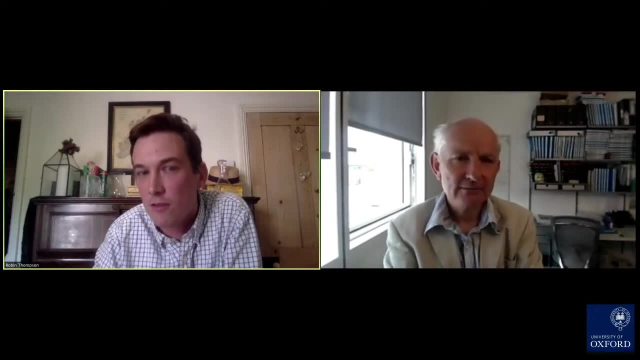 But do you think the 40%, Do you think the 40% asymptomatic transition would make a serious dent in the estimates of harm. So I think the 40% isn't a problem necessarily, because the 40% could correspond still to positive serial intervals. 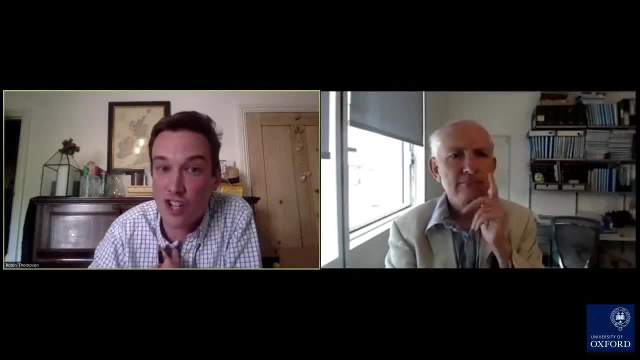 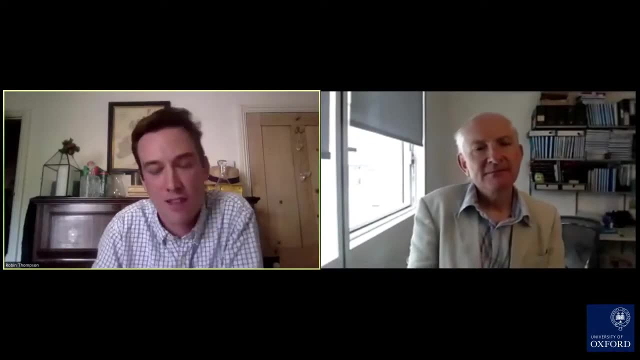 OK, So in other words, I could infect you when I'm pre-symptomatic, but then I could show symptoms and then you could show symptoms later. Right as long as That is all included. but it's specifically the negative serial intervals that isn't included. 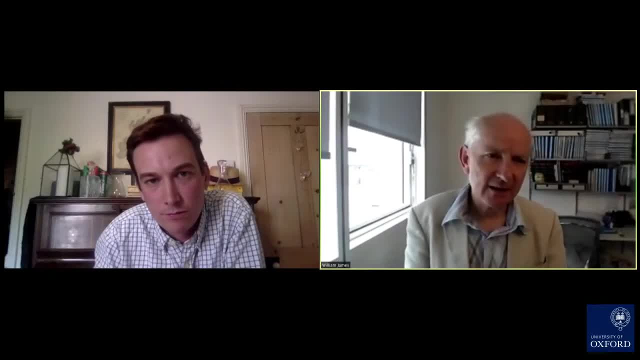 Very nice. Now we've had a couple of questions on the heterogeneity thing, which I think is a really interesting one. Anna Sue asks, and I'll try and get Sue's words right here. if I can find them, Give me a moment. 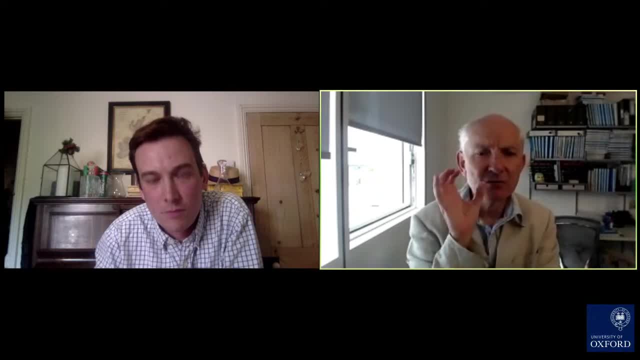 How much do these models account for the potential behaviour norms in each country, as opposed to say the population densities in each country? So that would be heterogeneity by country and culture rather than any other sort of thing. Is that a challenge? 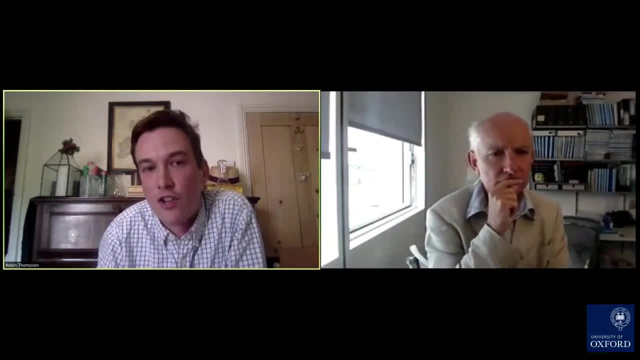 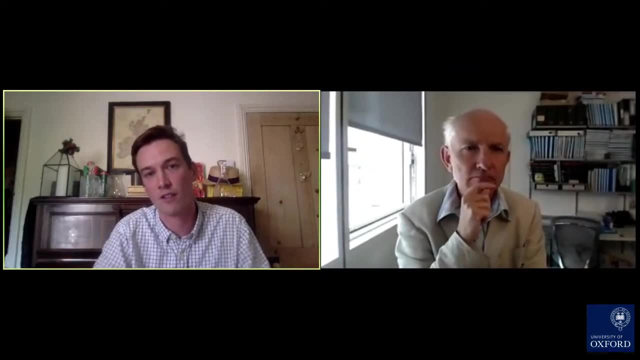 So that's something that is implicitly included in these estimates, because typically these estimates are conducted at the country scale. Sometimes these estimates are conducted at the regional scale. What we never do is take sort of all known cases of COVID-19 and estimate reproduction numbers. 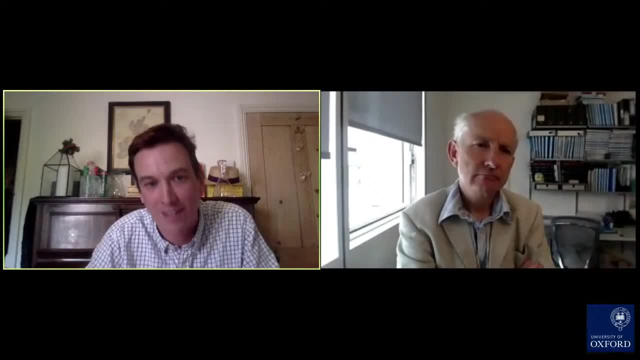 You know, those estimates wouldn't correspond to anything particularly worth looking at, I would suggest. So what we tend to do is we tend to take specific regions or specific countries and estimate reproduction numbers for that region or for that country, And thereby differences between countries are sort of implicitly included in the models. 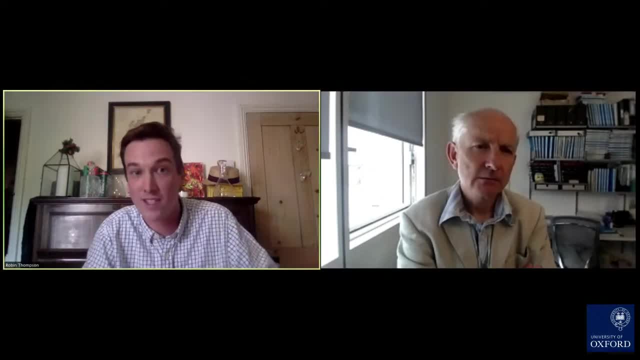 You can also have other models in which you explicitly code in behavioural differences. So those types of models also exist And that's something that certainly happens. But in the model I just described they're sort of implicitly there in the data and therefore implicitly there in the estimates. 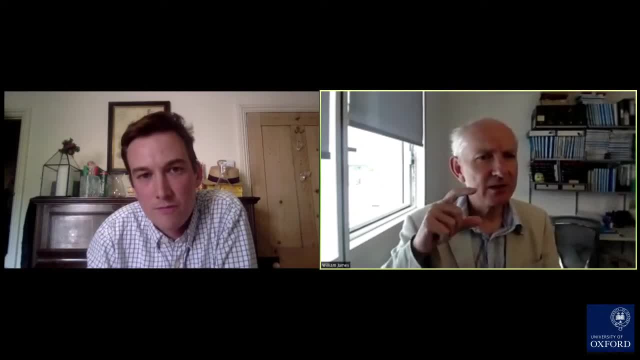 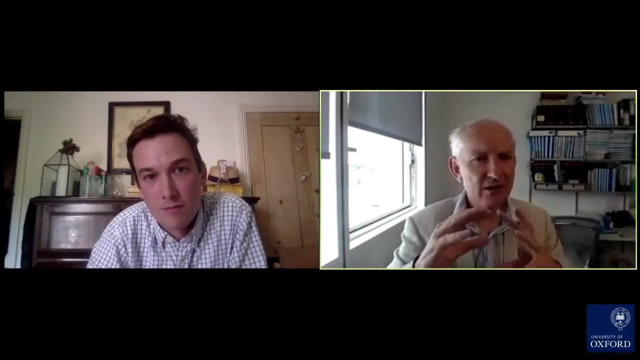 Although then I suppose Sue's question could then be rephrased in terms of communities within a country, because there's been a lot of discussion about certain communities Having different population structures, different socioeconomic standings, all the other sorts of things You could imagine being heterogeneity at community level within a country, couldn't you? 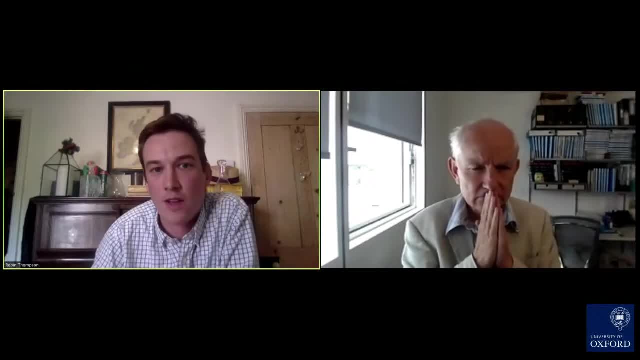 Yeah, absolutely Absolutely, And indeed there are models in which you have transmission through networks and the networks reflect the kind of spatial heterogeneity in the country. There are household models which explicitly sort of code in the fact that individuals live in households. 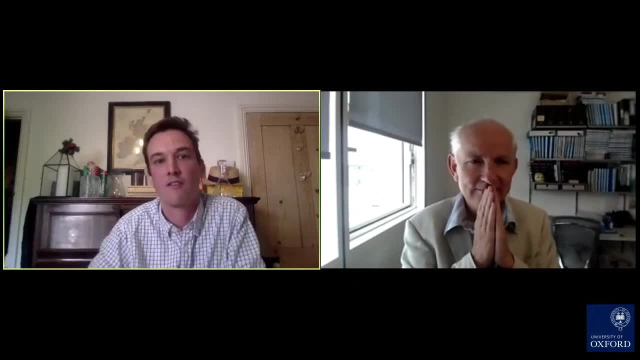 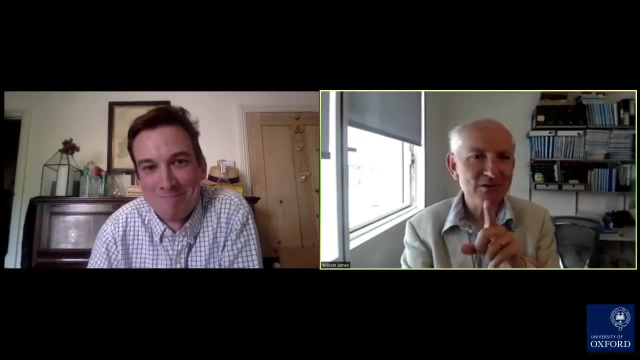 And so you get this local bulk up of cases and then transmission from household to household. Yeah, these sorts of things are very often included in models. Just the risk of digressing for a moment. That was something that interested me really early on. 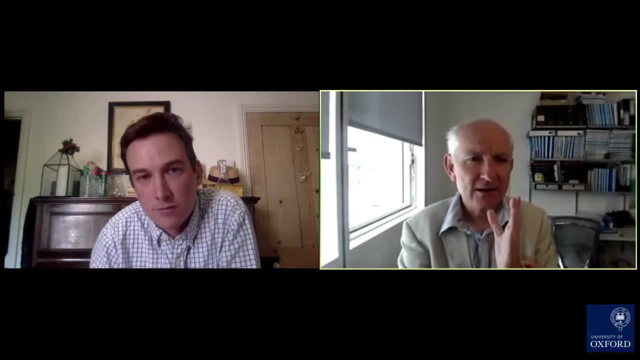 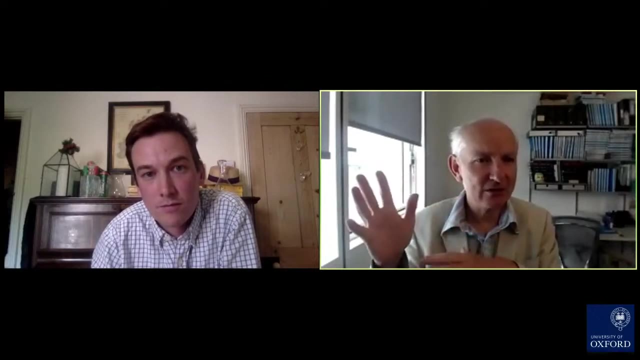 I don't know if I misread it all, But in the study from Wuhan, the WHO study, right back in February or March they estimated that 85% of transmission was happening in households and only a tiny fraction happening elsewhere. But then when we saw the imperial model coming out that was driving the government policy, 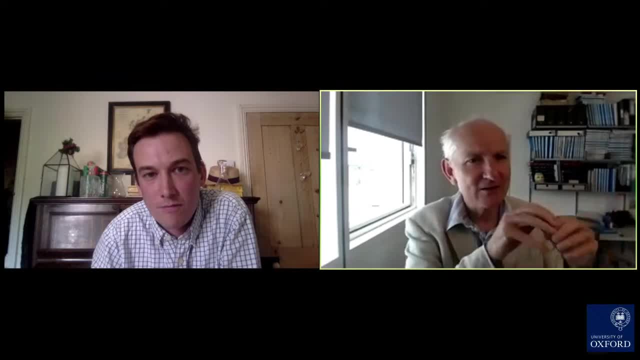 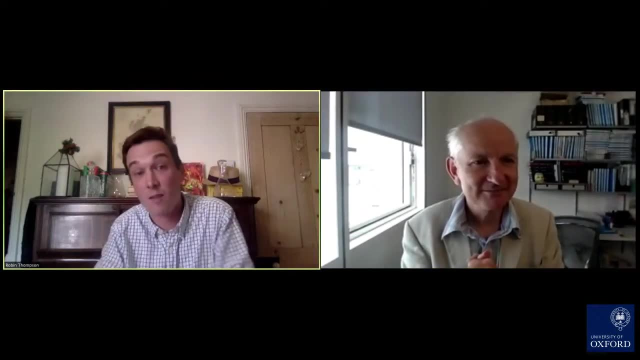 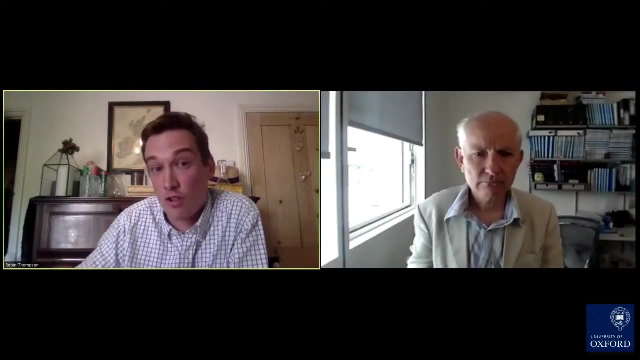 it made the assumption that one third of transmission was in households, One third in schools and one third elsewhere, And I wondered whether this was something that you had a view about. It's certainly something where more data would be massively beneficial. You can imagine that it also kind of follows on to so that different control interventions might be predicted to have very different effects. 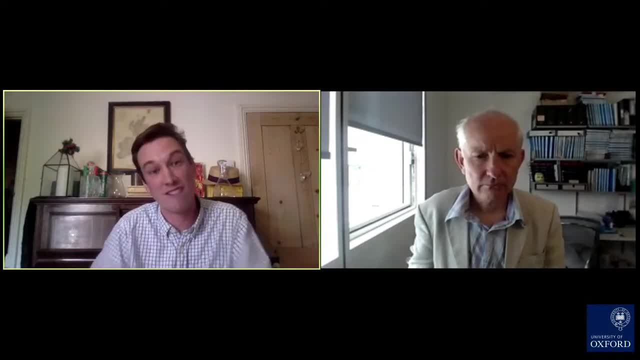 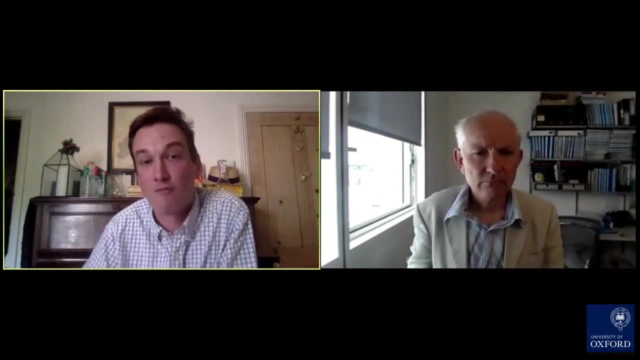 if you set the proportion of household transmissions to be very different to kind of school transmissions, Because, you know, something like a lockdown obviously puts people within households, thereby reducing between household transmission but potentially increasing within household transmission. So I think it's something where more data would be very valuable. 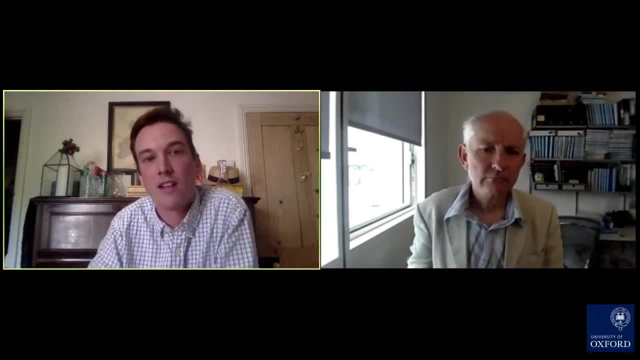 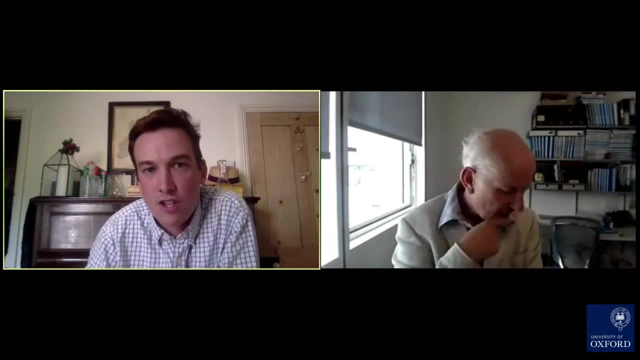 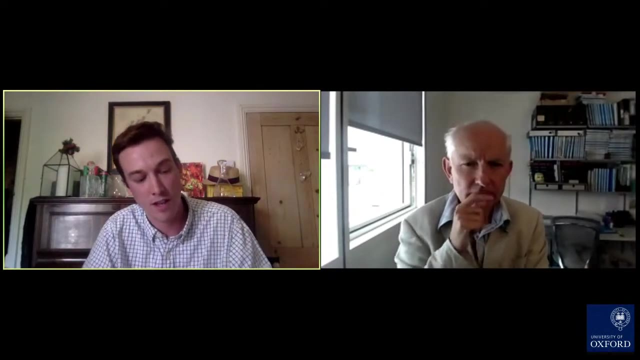 Something that has been measured, entirely aside from COVID-19, in a lot of detail are the numbers of contacts that we all have in different environments. So contact surveys have kind of taken place and looked at the proportion of contacts that we tend to have in schools or in households or, you know, in workplaces. 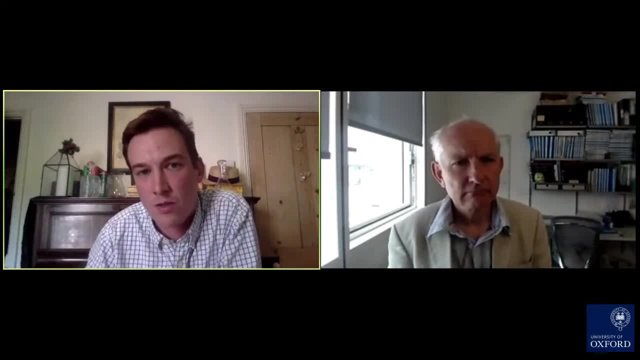 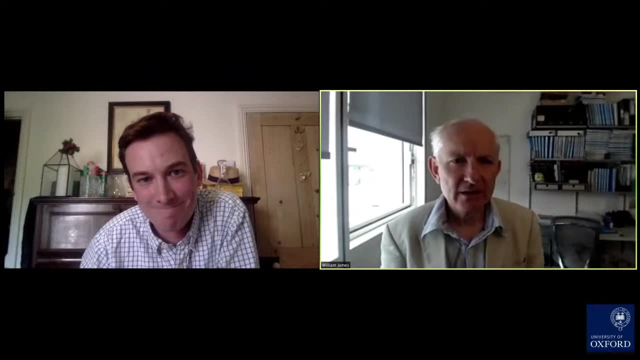 Or in other settings. And I think those contact surveys I assume were where the numbers in the Imperial study that you referred to came from, Right, OK, OK, that's great, That's very interesting. So just to slightly move away from the hard science, as it were, and into policy side of things, 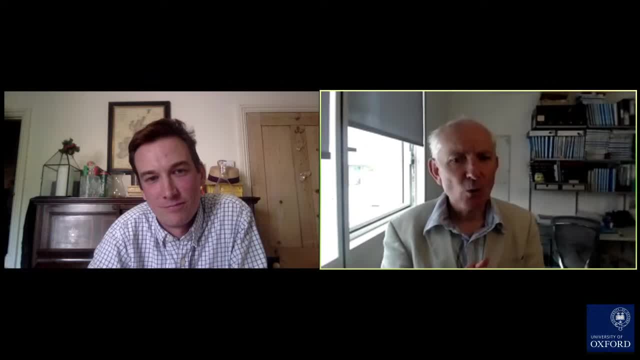 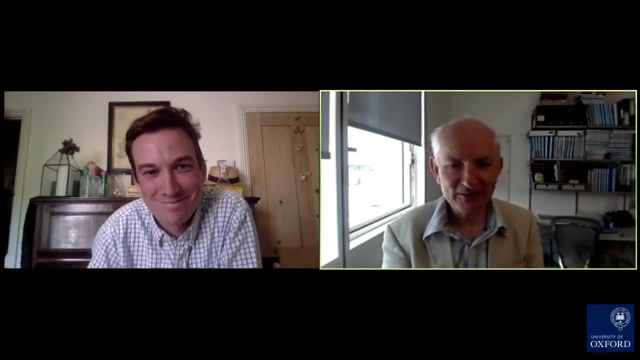 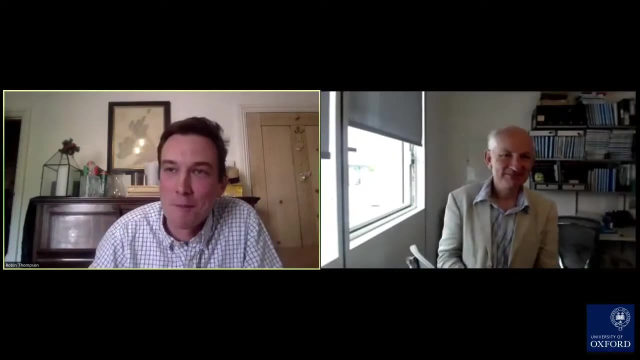 So Brian on YouTube has asked: when was epidemiology first developed So you can give us the water pump thing or something, And When did it first place in an outbreak? Yeah, that's a really great question. So yes, there is obviously the water pump thing. 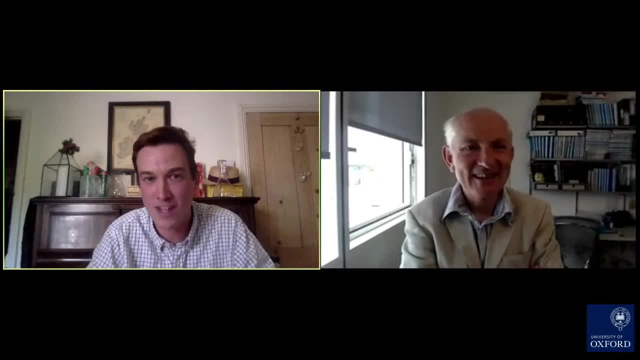 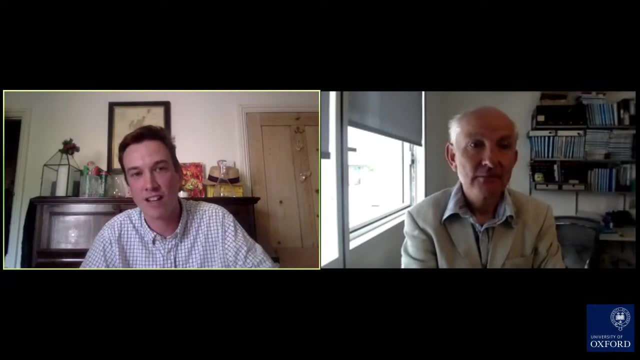 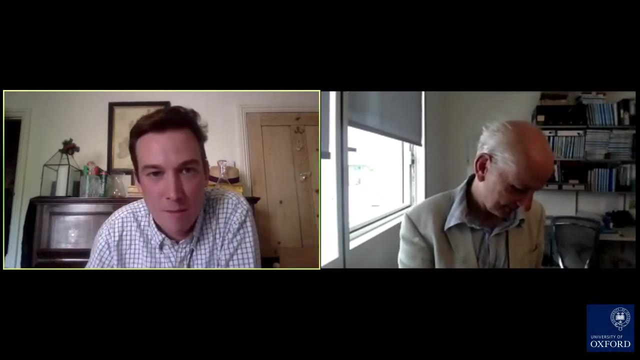 But I think the first example of mathematical models as we know them now. So these models in which you divide the population into different sort of categories. So you have infected individuals, you have individuals that are susceptible to the virus, And then you track the spread of the disease, sort of between individuals. 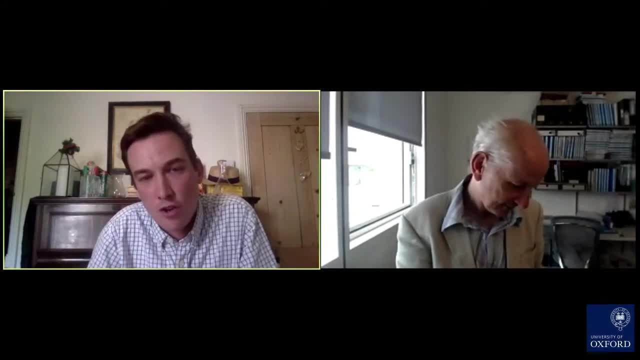 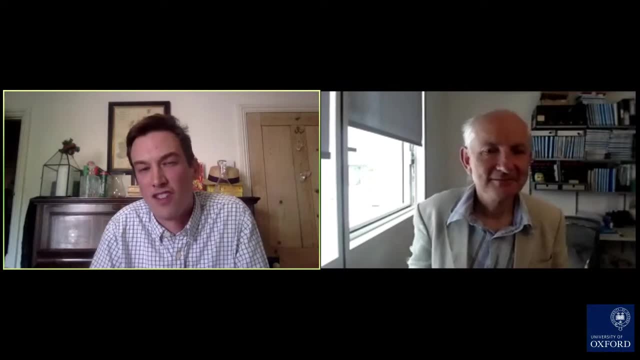 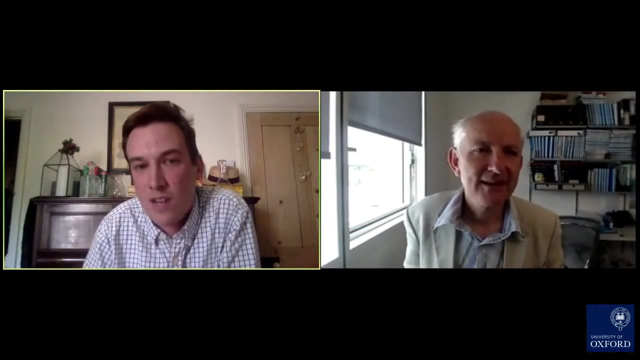 By moving individuals between those groups, Those types of models. So you know, one of the first examples was the models of Kermack and McKendrick in the 1920s And kind of shortly before that. So really I would say it was the beginning of the 20th century that the kind of research field really took off as we know it today. 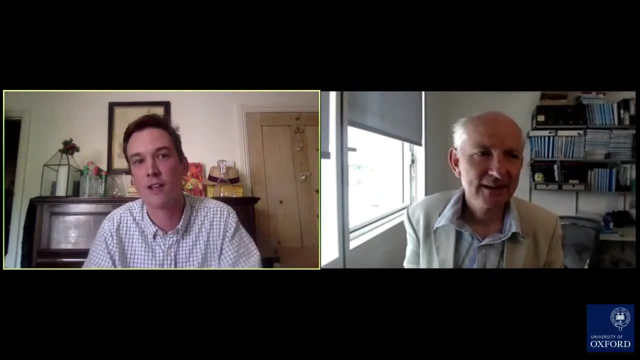 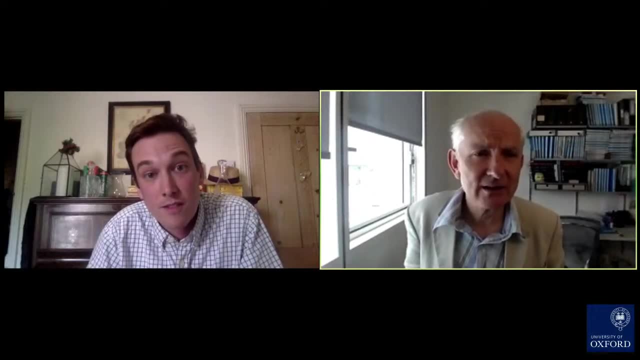 Where what I'm talking about really is mathematical epidemiology rather than epidemiology. Exactly, Yes, It's quite a long history. I think many people think it's really recent, but actually it's quite a long history then, isn't it? 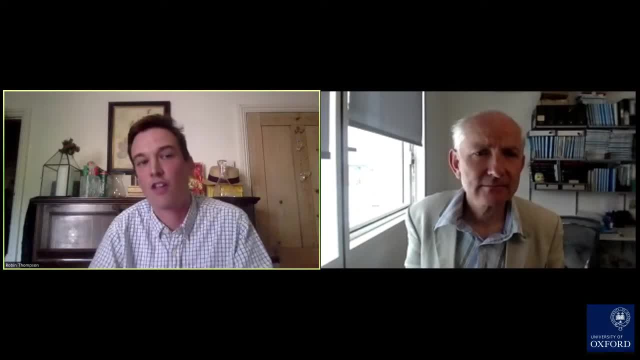 Yeah, absolutely Absolutely. The thing that is more recent, though is the kind of very recent thing, is that the real time use during outbreaks to guide control measures. So in the UK the first use that I'm aware of it directly feeding into policy is the foot and mouth disease outbreak in 2001.. 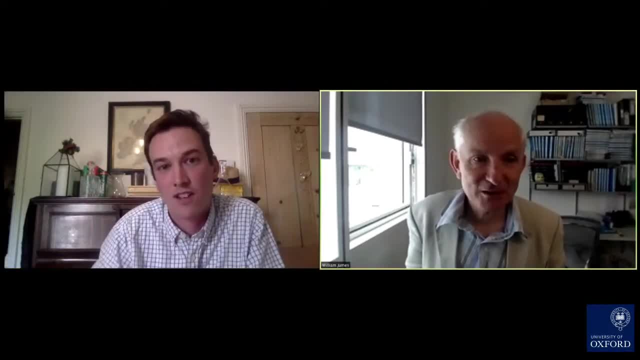 So there it played a really big role in precisely where I think the Imperial model was used. there wasn't it. And again, Imperial, Yeah, yeah, exactly. And in fact there were kind of several models all used at the same time. 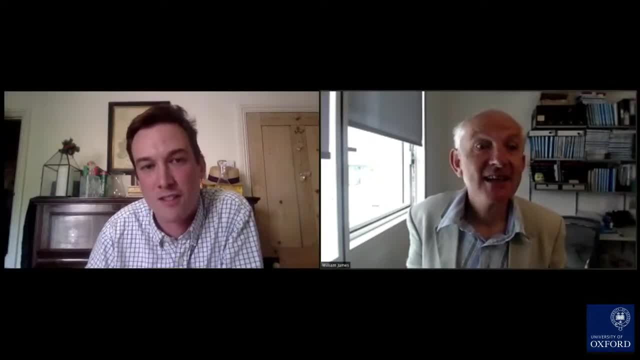 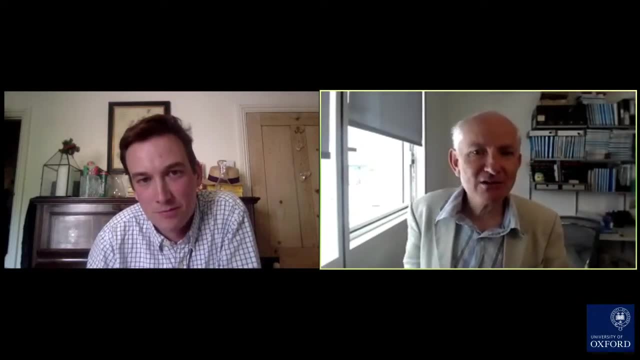 But Imperial was one of them. There's one from Warwick Very good. Well, relating to that, Margaret on Facebook asks: do you think governments worldwide have been acting in response to the models they've been presented with? too much or not enough? 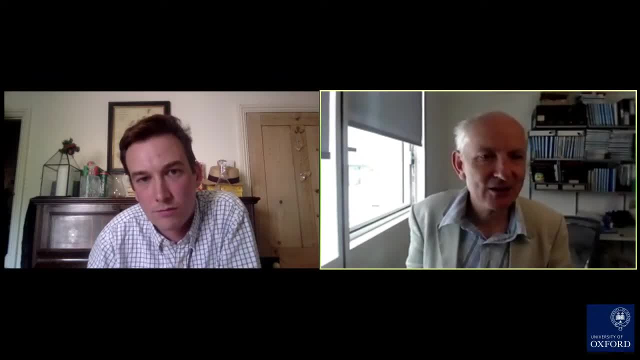 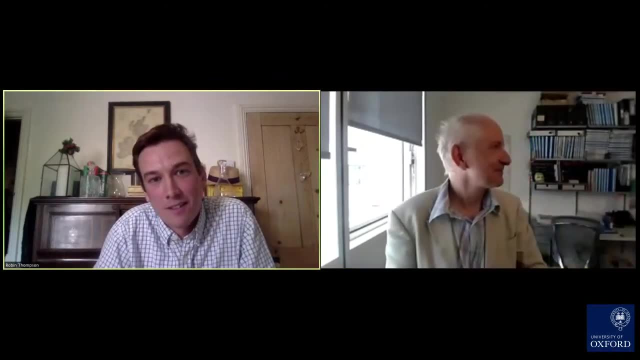 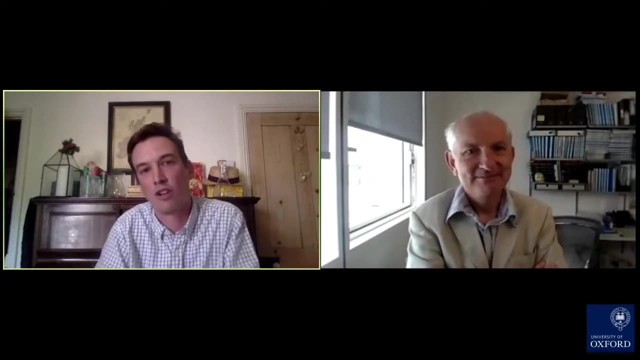 So how well have these models been deployed in your view? Governments worldwide- That's a very big thing, isn't it? So yeah, absolutely That one. So I think, certainly my own experience, My own experience is- is that there has been a lot of interaction with modelers. 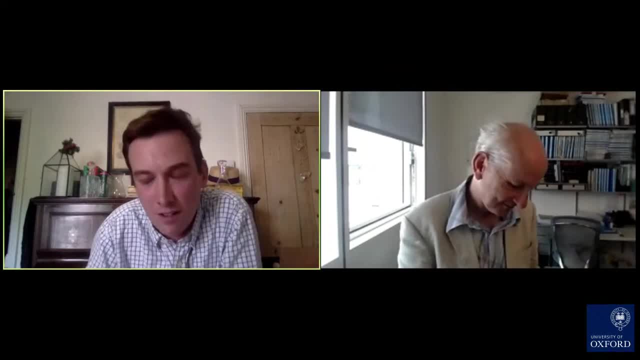 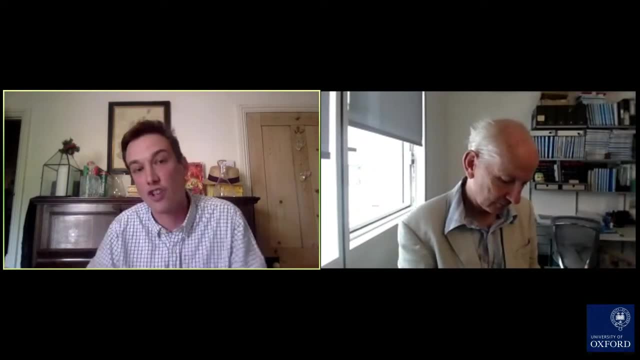 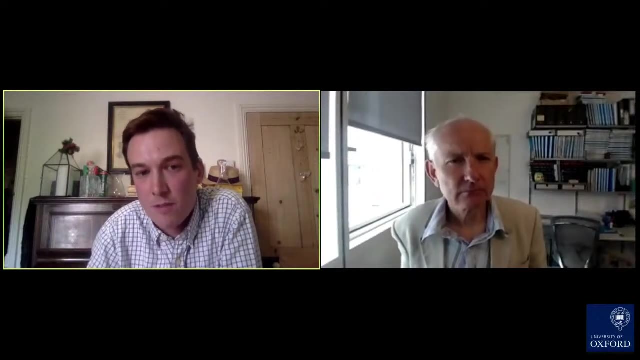 And so actually bringing the lockdown in in the first place was, as has been widely reported in the media. You know, one of the key inputs for that were modeling predictions predicting huge numbers of individuals that were likely to become infected. So in the UK I think, yeah, we certainly have been responding to modeling predictions, particularly at the beginning of the outbreak. 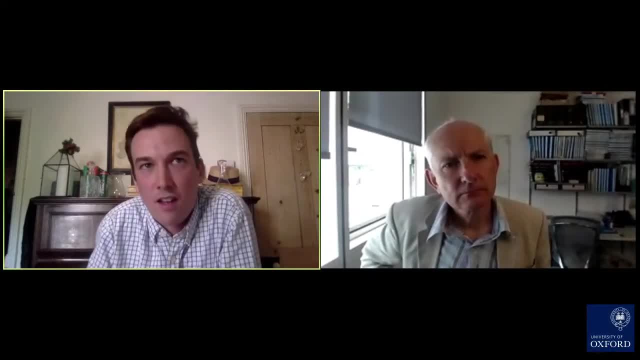 But more widely across the world. I think something that is a really big issue at the moment is actually there are lots of countries without the modeling expertise for models to be developed there to then be kind of fed into policy, And I think there's a huge responsibility for modelers in countries where there is a substantial amount of modeling expertise in places like the US or the UK, to actually provide support particularly to lower and middle income countries to then actually feed into government policy in those places. 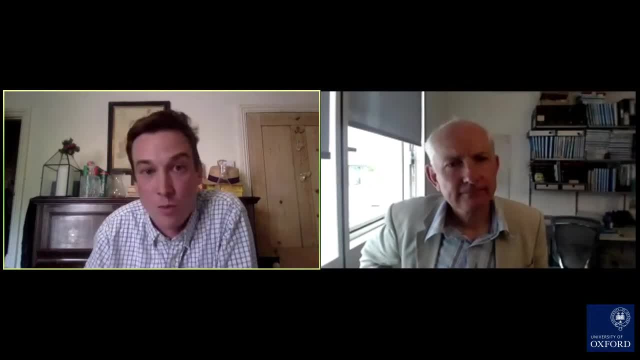 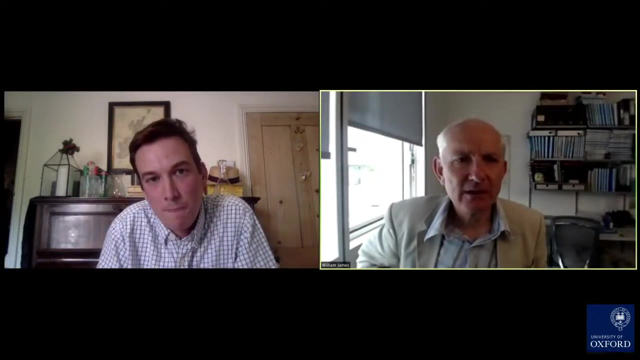 And that's kind of funny. TTYs think we have most places, Very few, Very few countries in the world. Right, The delivery process would have been more cœ, momentarily lower than Yeah Right, could the who have a role in that? do you think yeah, absolutely, absolutely, and i think, um, i think. 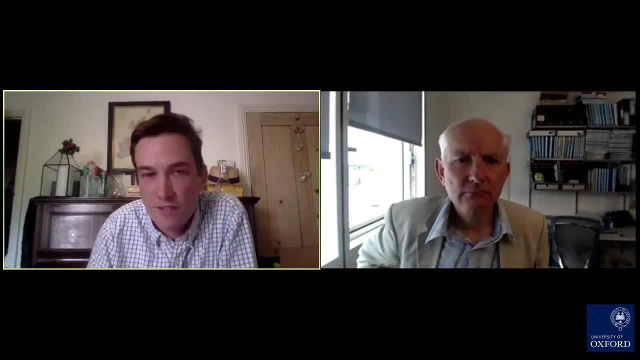 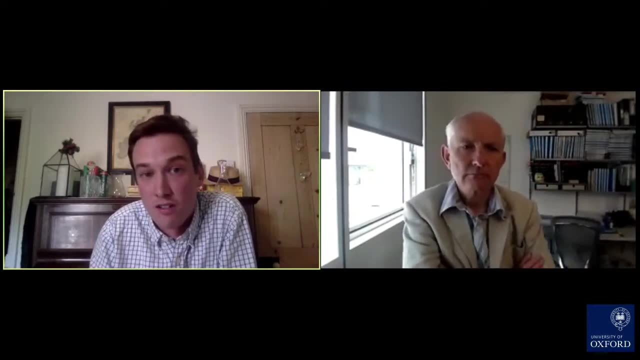 they, they do a great job in that respect. so, in fact, um, you know, i've done some work with uh individuals at who before looking at ebola, and they certainly interact a lot with modelers in the uk and elsewhere. so, yeah, they have an absolutely huge role now. paul on facebook asked. 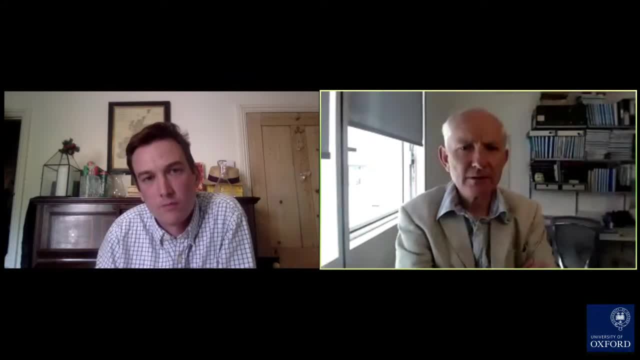 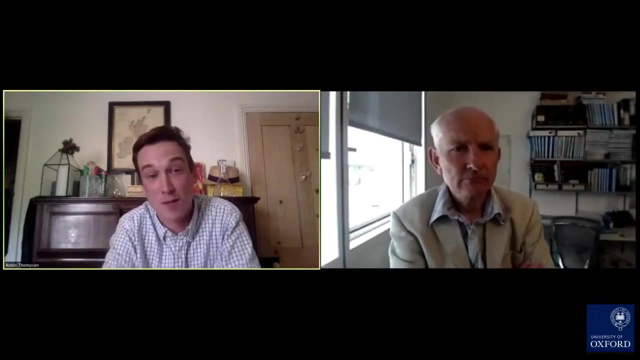 a question that i think you might you might have addressed, but worth worth just checking. so he he wonders whether um rrt should be the major way that governments decide on the actions they take. if not, what else should they consider? that that's an absolutely fantastic um question. so rt is one. 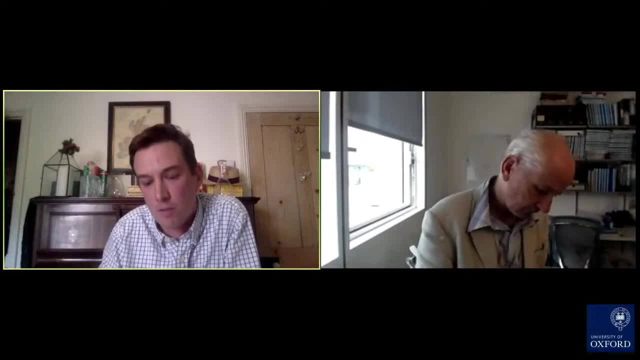 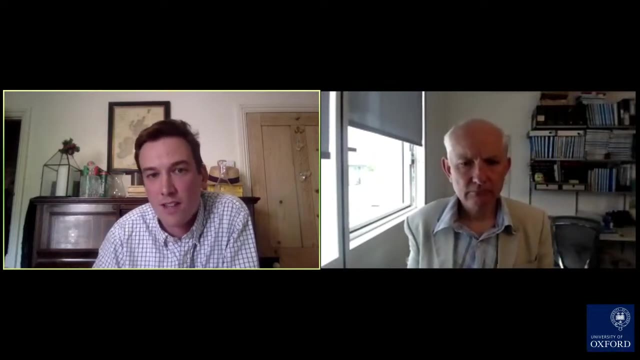 metric, but it absolutely is not the only metric that should be tracked throughout an outbreak. so, in particular, what the time dependent reproduction number tells you is it tells you whether or not the outbreak broadly is under control. so if, um, if rt is bigger than one, then you would expect case numbers to kind of take off, and if rt is less than one you would expect 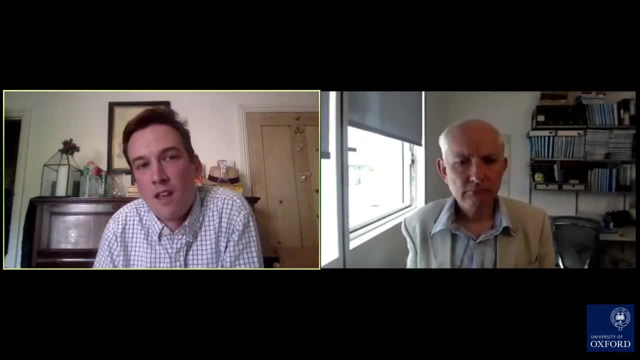 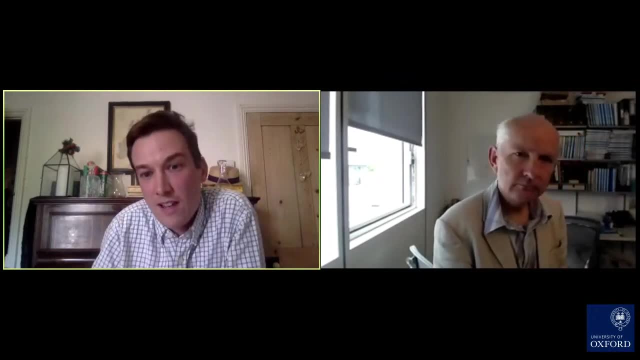 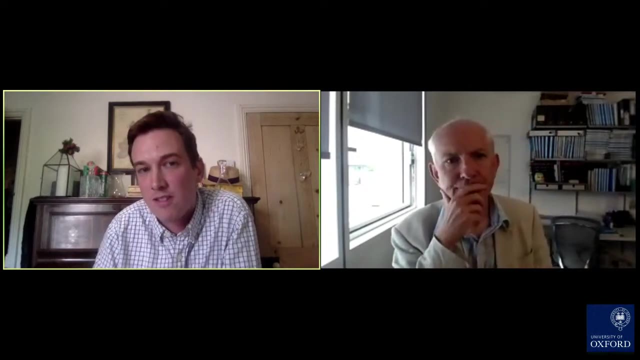 case numbers in the long term to decline. um, what it doesn't tell you, though, is how quickly that's going to happen. so if you imagine the case at the moment in the uk, so case numbers are relatively low, and the thing that we're worried about is a surge in cases. if that surge happens, how quickly? 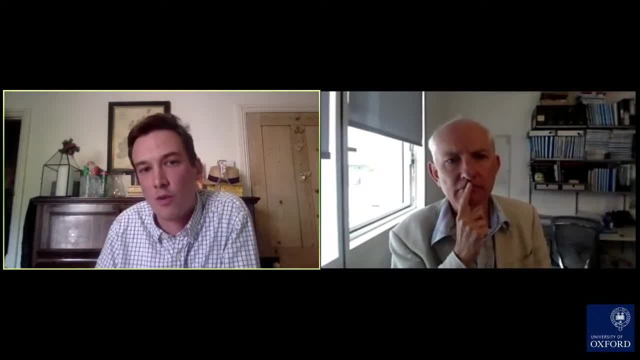 that surge happens is something that's very important, and so, in order to figure out how quickly that surge happens, rt will tell you that a surge is going to happen in the long term if it's bigger than one, but how quickly it happens relies on you looking instead at epidemic. 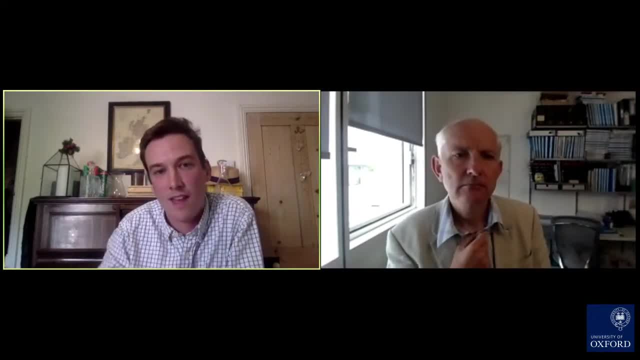 growth rates. so, in other words, looking at numbers of cases and how quickly the epidemic ends up taking off. um so rt is definitely something that should be tracked, but there are other things that should be tracked too. so i would say overall- there are basically three metrics- that it's very. 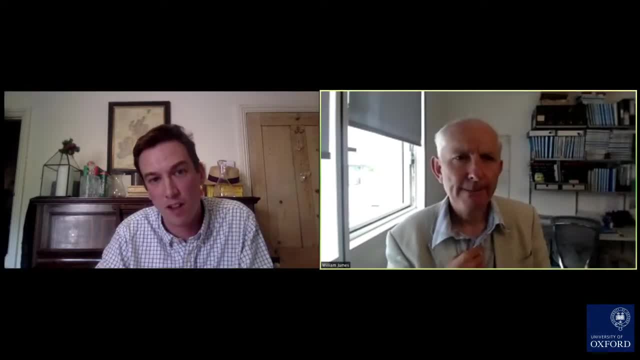 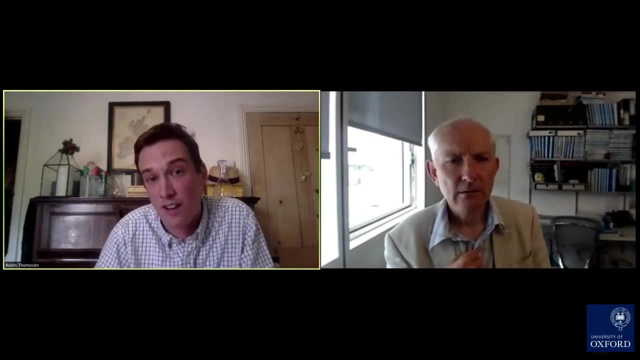 important to track. one is the time dependent reproduction number, yeah. another one is the growth rate. and then the third thing is actually just numbers of cases or numbers of deaths, and the reason that that's important is, you know, for example, if the reproduction number is one case numbers will remain pretty much flat. 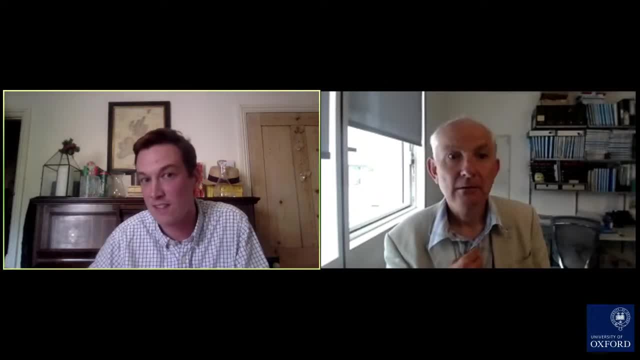 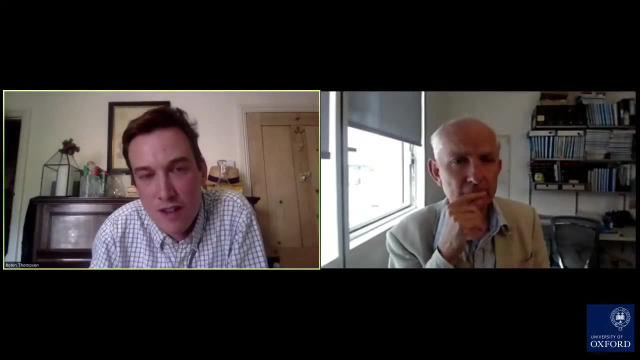 it's very different if the case numbers are very low and it remains pretty much flat. the case numbers are high, absolutely much flat, yeah, um so. yeah. so i would say they're kind of three of the main metrics to track during almost any epidemic and i guess, following up with that, 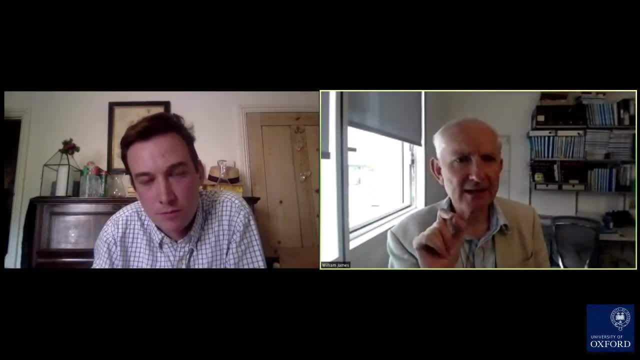 this. this kind of gets into the next question i'm going to ask you. i guess the ascertainment is really important, isn't it so? particularly when you're at a low base. uh, knowing how many new cases you've got requires an awful lot of sampling, doesn't it? yeah, absolutely, yeah, absolutely and actually. 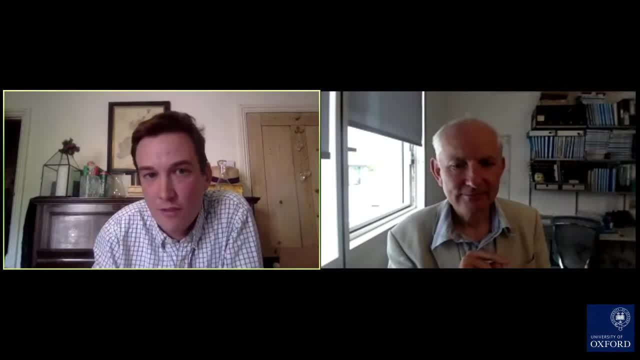 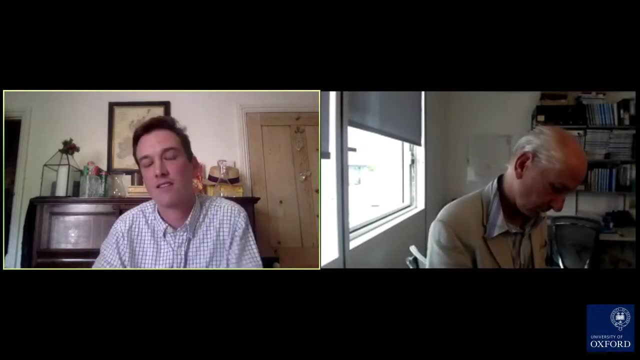 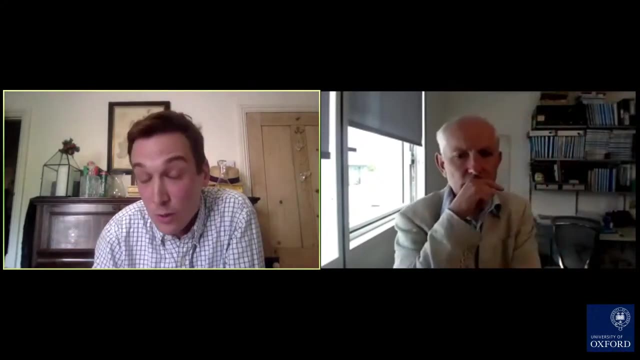 estimates of the reproduction number depend very significantly on sampling, because if you imagine you, you know you sample more people, you detect more cases. it's pretty hard to to sort of unpick that from an actual increase in in transmissibility, um, so yeah, so that's, that's also a really 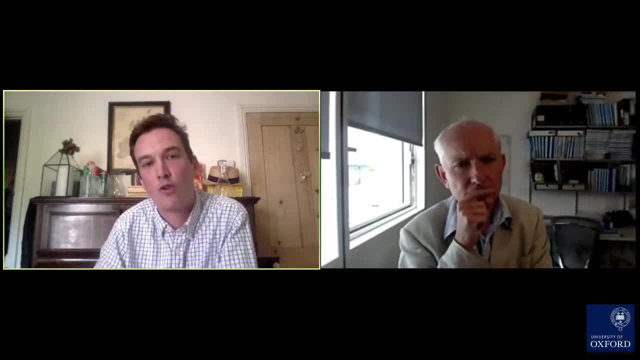 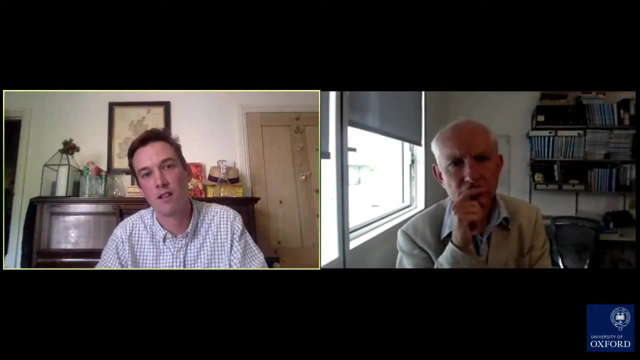 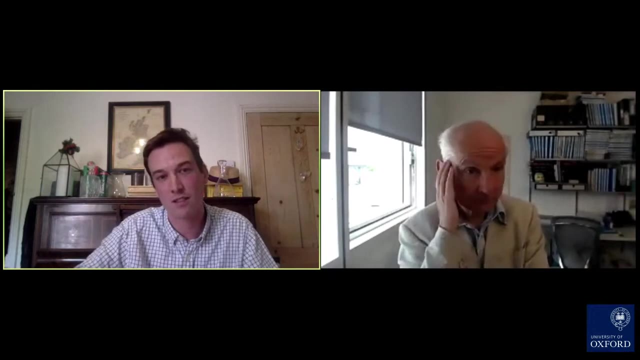 interesting point. one thing, though, to note is that if your level of testing remains constant, if you're detecting a constant proportion of all cases, then reproduction number estimates are very robust, because actually, going from, you know, 500 cases to a thousand cases might indicate a reproduction number of two, and that's the same as if you detected half of all of those cases. and 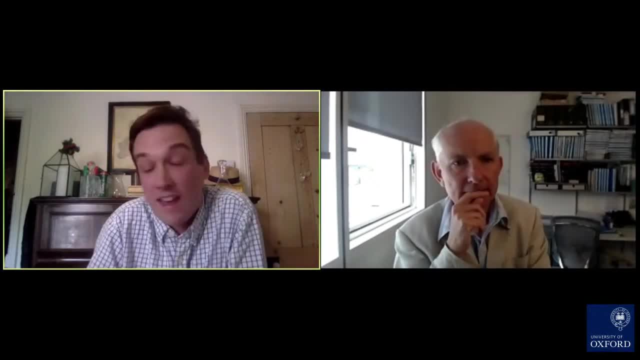 went from 250 cases to 500 cases, um, but yeah, so certainly going forwards again. i think something we can- we can massively learn from this epidemic and previous ones- is actually keeping track of and actually building that into estimates of of the reproduction number, um, another thing you can do. 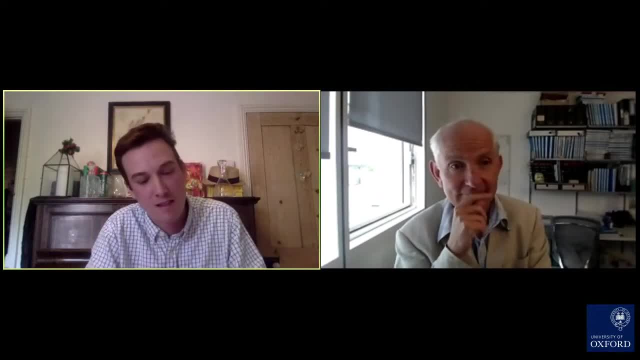 though is, you can also look at other data sources so you can look at, for example, number of deaths through time and estimate the reproduction number using um, that data too, and that data is likely to be a little bit more robust to to um, precisely how many individuals be tested. absolutely so, csk. 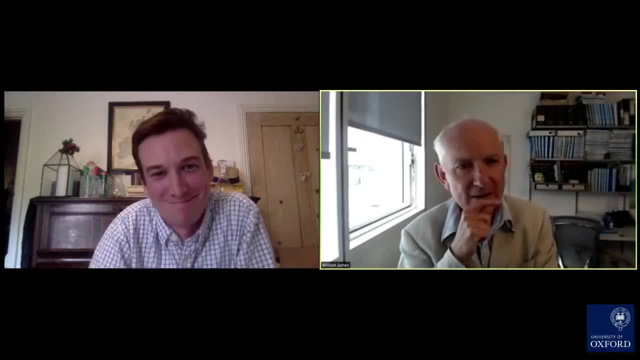 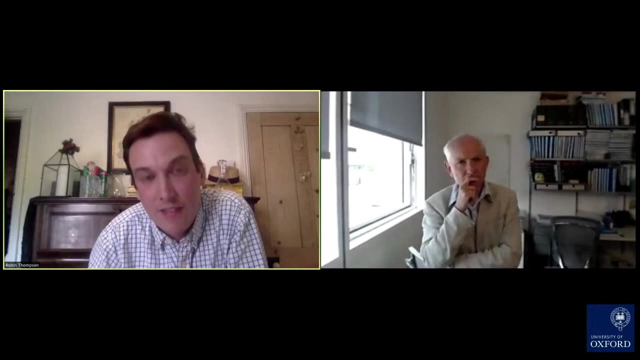 on youtube. um, uh, asked a question about testing. um, what about serological data testing? would that be useful to you? does it give you extra information, or is it? is it not really the stuff that you need for your input? yeah, yeah, it's very useful, and the reason the reason it's very useful is that gives 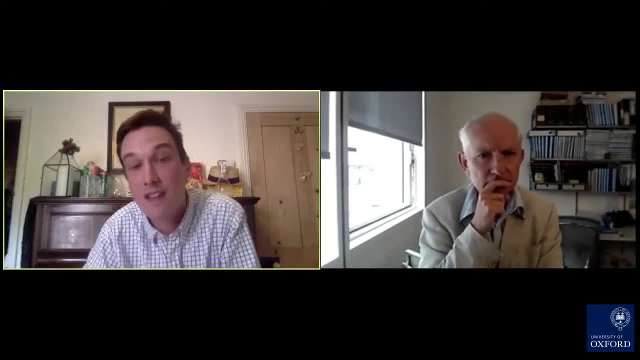 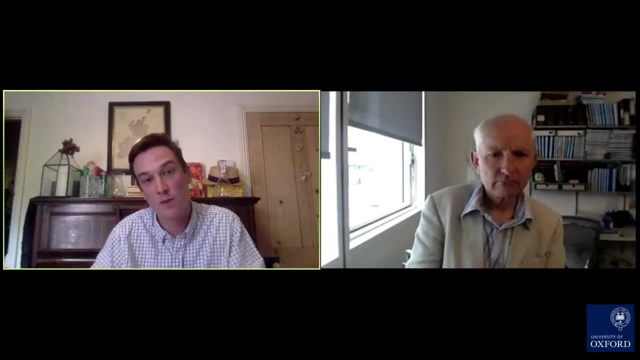 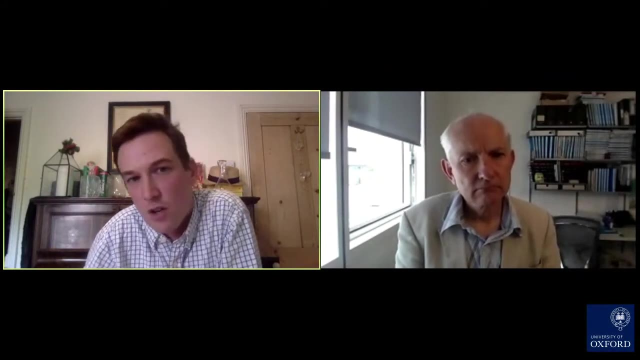 you an indication of how many individuals in the population have previously contracted the virus and then may potentially um be immune, um, if that number is very high. so if you have a large number of immune individuals, then that lowers the reproduction number, um, because there are fewer kind of targets for infection. and so, yeah, again, again, that data is is extremely useful for sure. 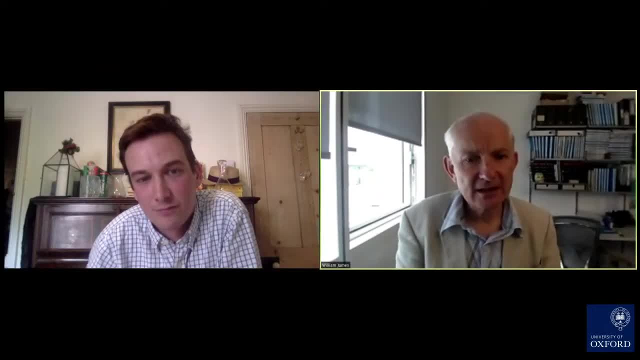 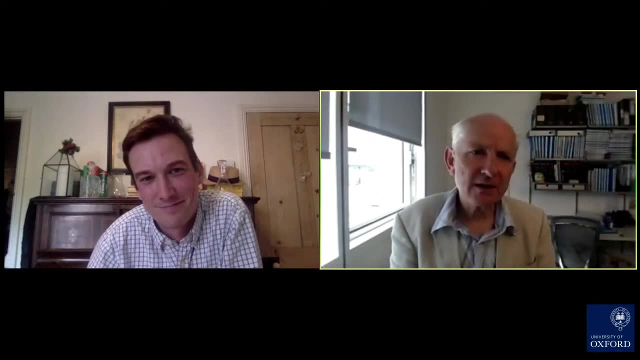 now charlie on facebook. i think charlie's asked: oh, there's several charles's and charles uh asking questions. it's, it's the. it's the right name for this. um, in terms of the interventions, the non-pharmacologic interventions, um, have you taken a view of the analysis on the utility or otherwise? 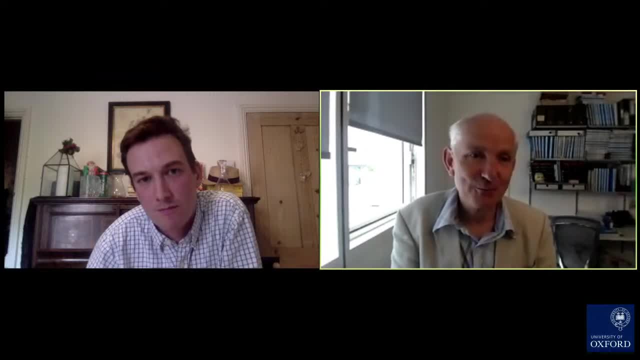 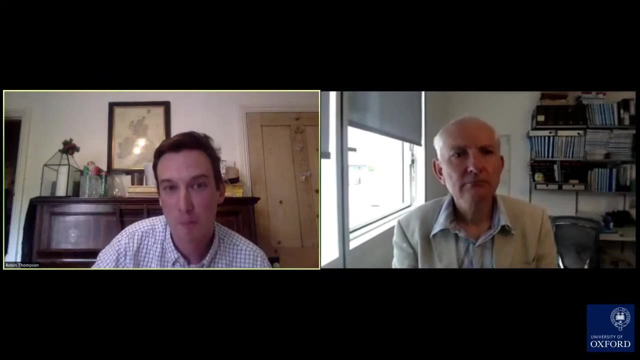 of face masks as an intervention. it's obviously a very hot uh topic, uh, at the moment. there have been a couple of things relatively recently in the press about this. what's your view about the quality of the analysis? um, so i think you know that's certainly that's not something i work on personally, so i haven't. 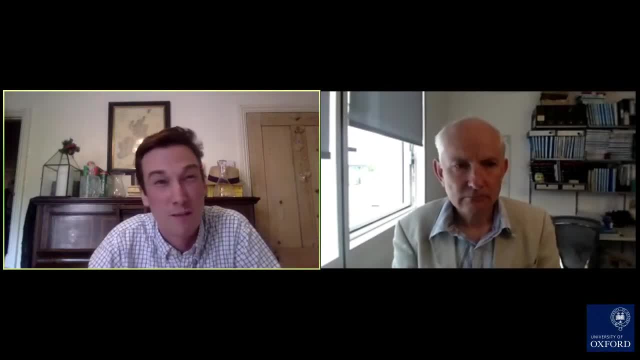 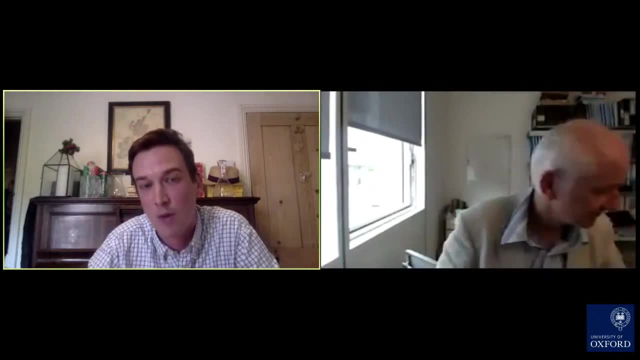 conducted any analyses myself about how effective face masks are. i guess my viewpoint on it generally, though, um, is that if it is going to make a difference, uh, to the reproduction number, if it's going to lower it even slightly, even if there's any chance that it will lower it even, 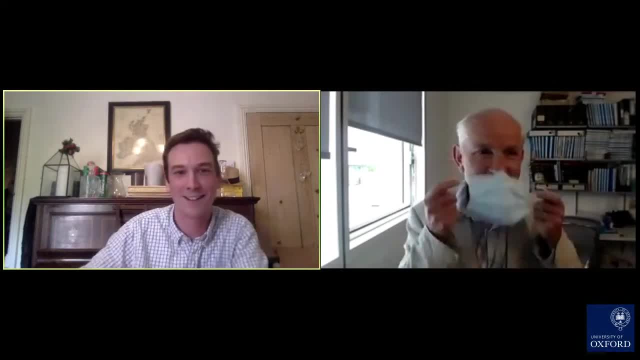 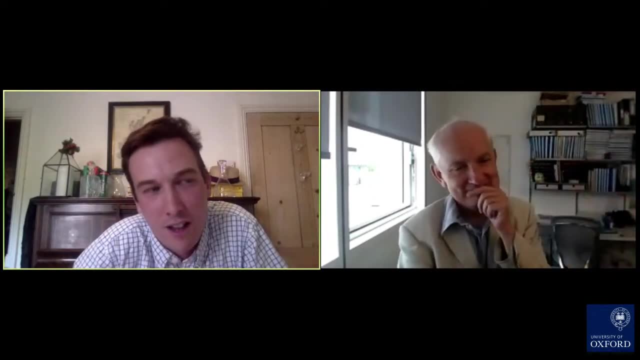 slightly, then you know why. why would we not choose to wear exactly? i've got mine here too. there you go. so yeah, what? why would? why would we choose not to wear face masks? um, i guess the only thing that should be that you should bear in mind is that, if you are 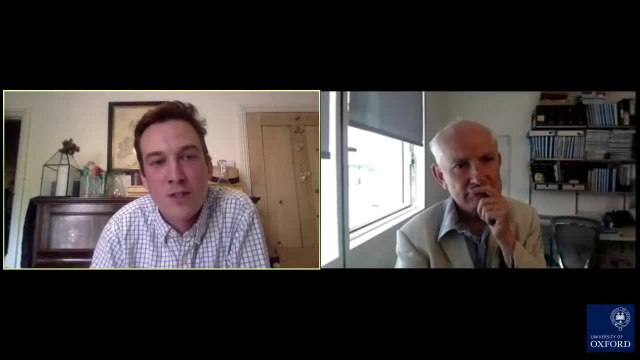 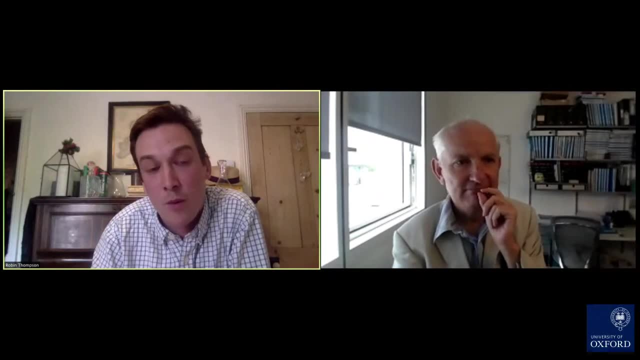 going to wear a face mask. um, that shouldn't sort of give you permission to act any differently. but yeah, the effectiveness of face masks isn't something that i personally study, but you know why wouldn't we wear them if it was going to have the chance of reducing the reproduction number? 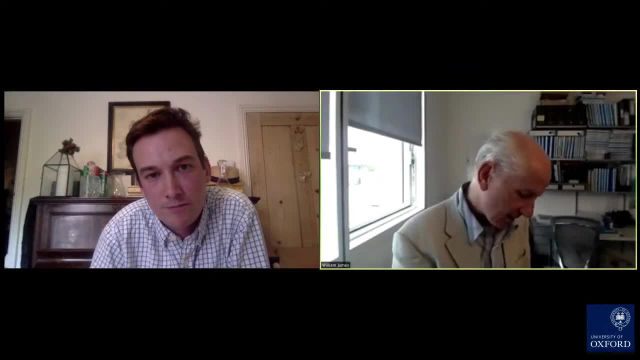 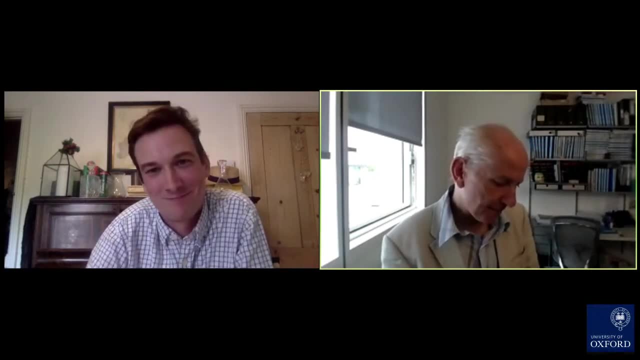 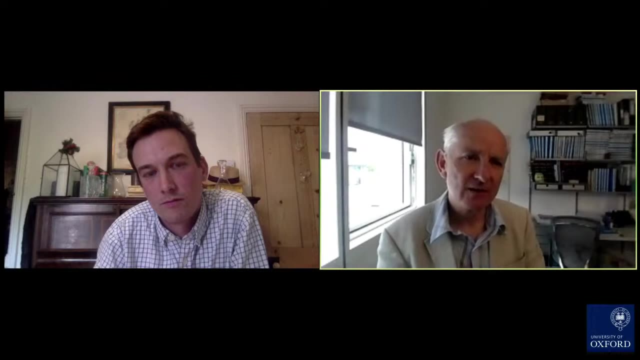 exactly all right. so, um, i think now we get on to the slightly, um, uh, broader questions. only a couple of questions. um, brian is asking: what do you, what do you feel about the general quality of discussion of this sort of top of the epidemiology and mathematically epidemiology topic in the general? 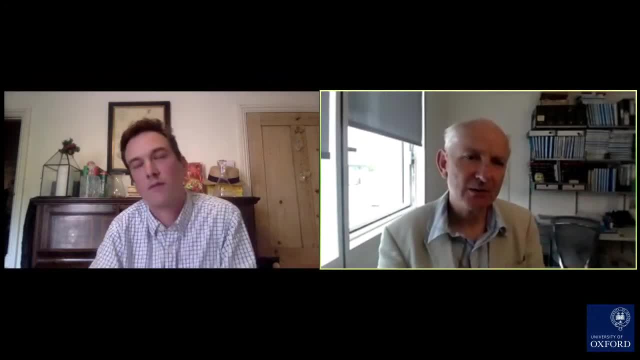 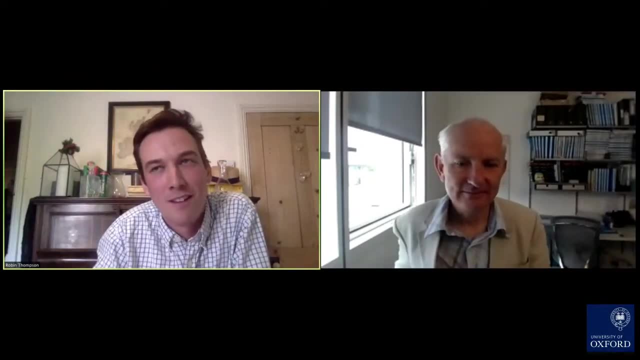 media. what's what? what's your reflections on that? you must, you must see a lot every day and react to it. yeah, um, yeah, absolutely. i mean. i guess the first thing to say is that, um a year ago i i sort of never expected, um, that mathematical epidemiology would be in the media as much as it. 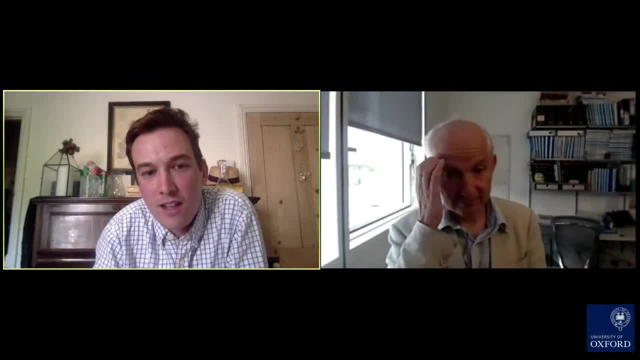 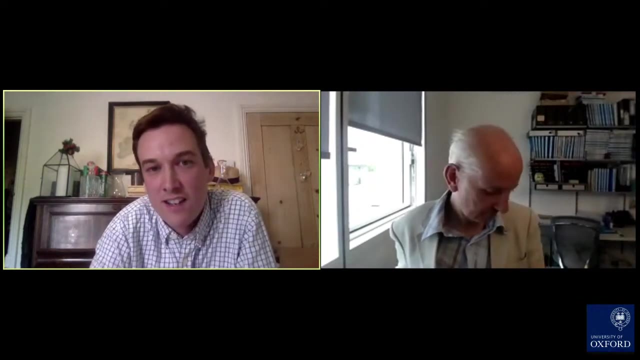 i think, broadly, the reporting is pretty good. however, the one thing that needs to improve, in my view, is um how uncertainty is reported. so in particular, you know people don't really like- and policymakers in particular don't don't particularly like it- if you tell them that the reproduction 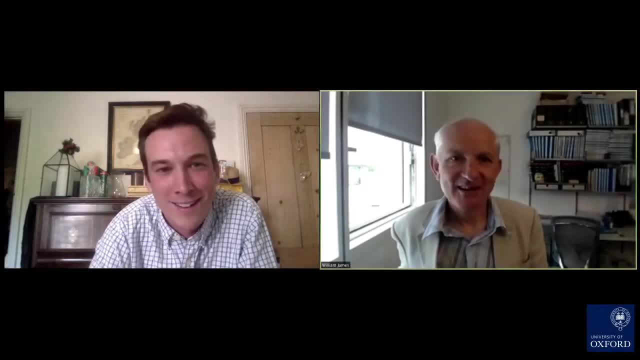 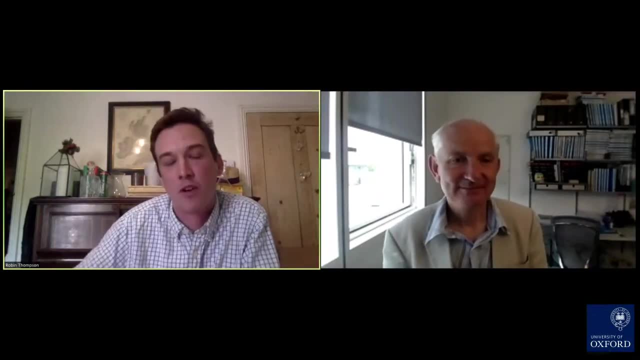 number is two, but it could be anywhere between 1.2 and three. um, yeah, people don't respond too well to that, but actually that uncertainty is very important because it tells you about the range of possible outcomes. and it tells you about the range of possible outcomes. and it tells you: 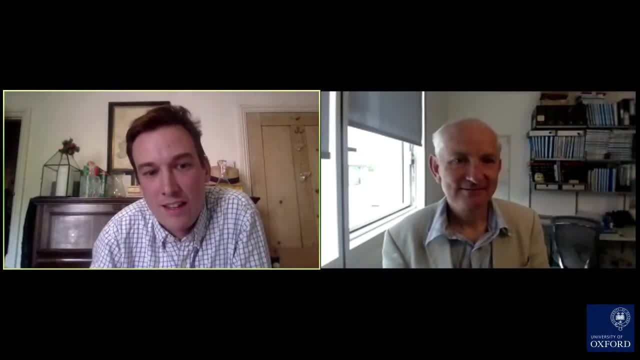 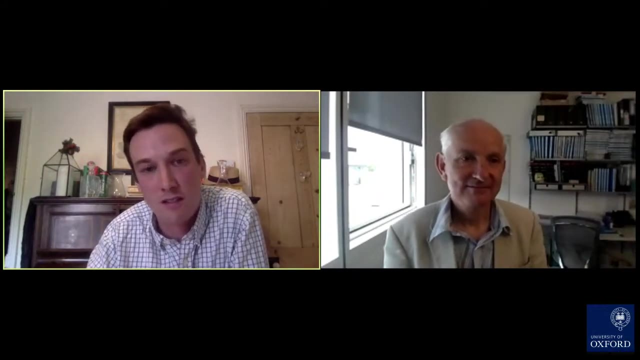 um, and the one thing that i would strongly uh encourage um modelers to do better is to communicate that uncertainty um to journalists and policymakers and in turn, i would hope that those individuals would would go on and um and sort of communicate that uncertainty to the wider. 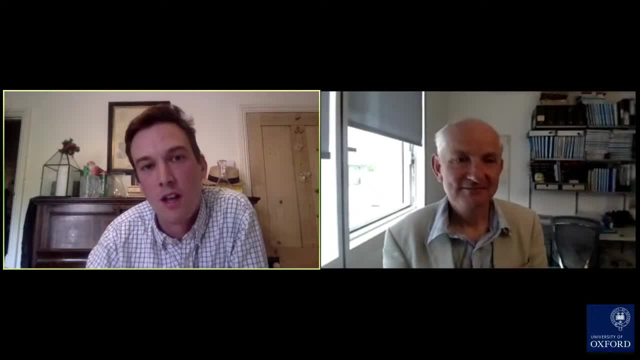 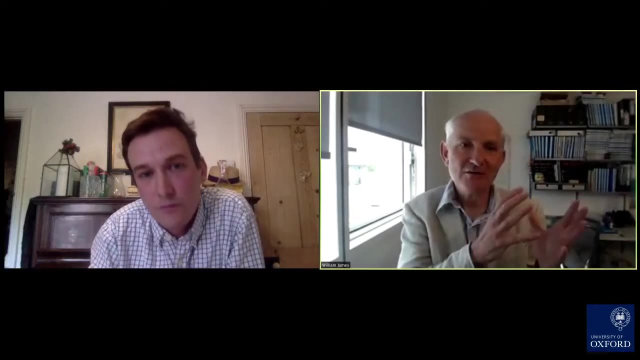 public. so i would say it might be that's the biggest current issue, um, but you know, i think the fact that uh, concepts like the reproduction number are being communicated to the general public is really a good thing. i, i totally agree. so you, i mean, you've done, you've done a good job. 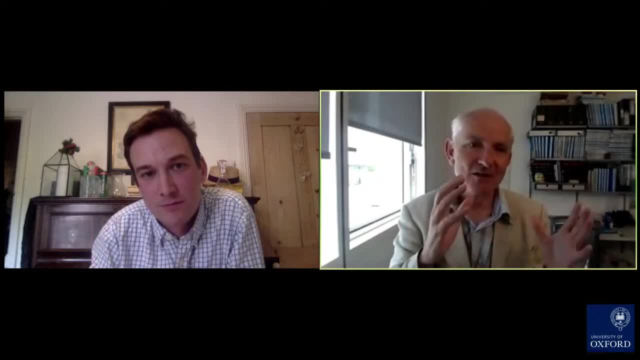 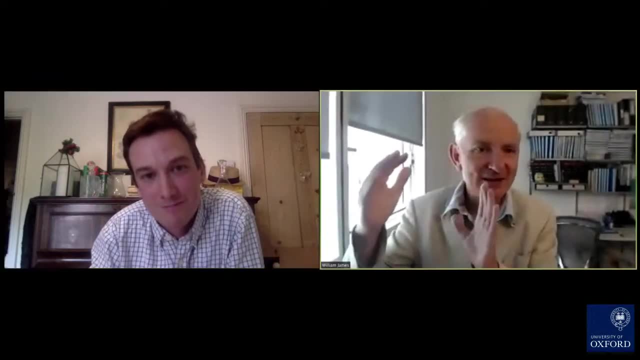 today. so far in in in getting people to think about those quantities as opposed to the qualitative. yes, no sort of things is what most people like to think about, but on top of that, thinking about the uncertainty bounds is a really important um uh piece to piece to play into it, which i think. 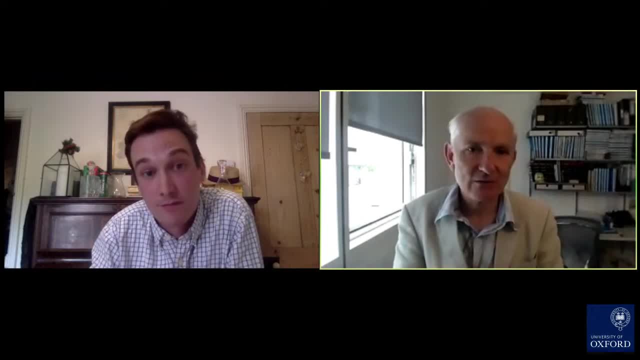 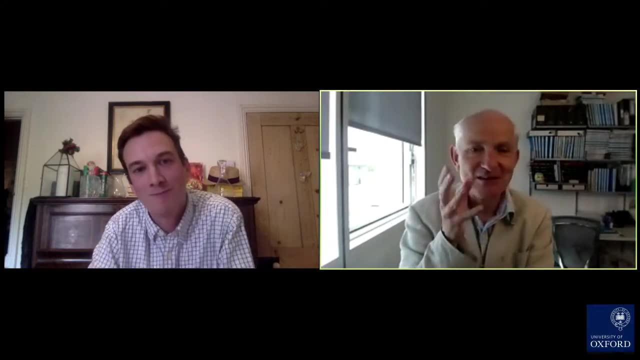 we all have difficulty with, and so it's not surprising it's a challenge for the general public. well, the last question, um, uh, which is the question is: do we have a way of thinking about on the public side of things? i like this one. i just had to bring this one in from jenny on facebook. 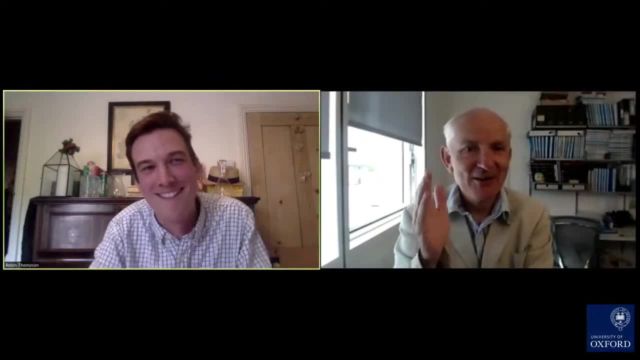 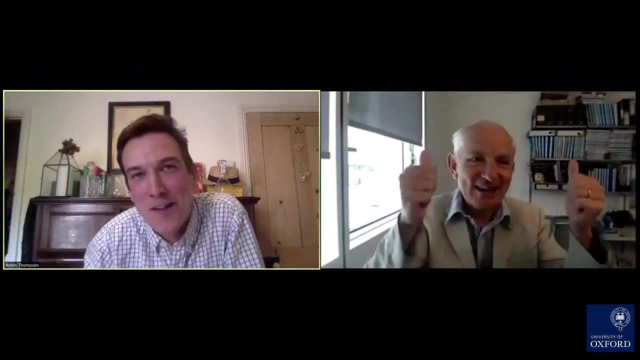 have you seen the film contagion? what did you think about the way the r number was described in that film? please don't tell us you haven't seen it. i have seen it, i've. i've been trying to avoid watching films like that, though. since the beginning of the pandemics, so it's quite a long. 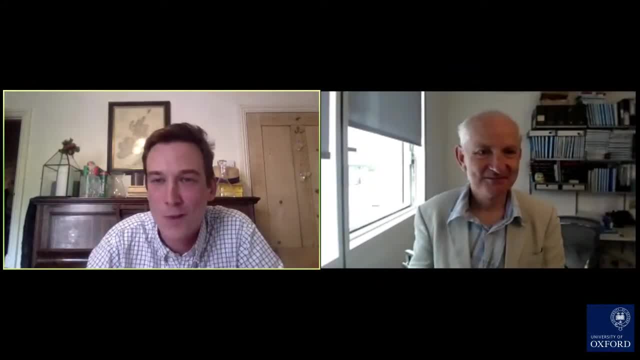 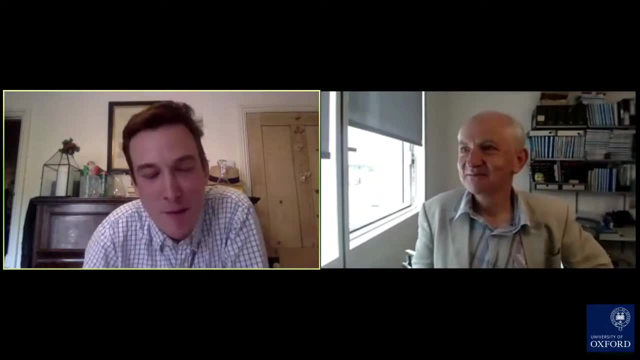 time ago, um quite a long time ago that i saw it um, i guess within mathematical modeling or within epidemic modeling circles. i guess it's obviously very well known because the r number, um, is depicted in it and obviously now the r number has been depicted in in kind of so many different. 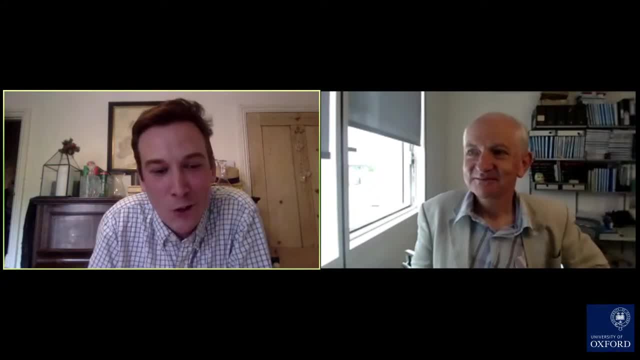 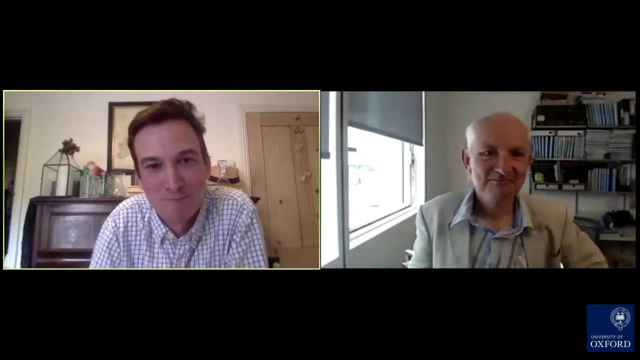 places. so uh, so yeah. so i think, um, again, it's kind of good that that concept was was depicted, but but now it's maybe uh out there more widely in the public than it was before. well, robin, that was a really fantastic talk and thank you for answering those questions so well. i've, i've. 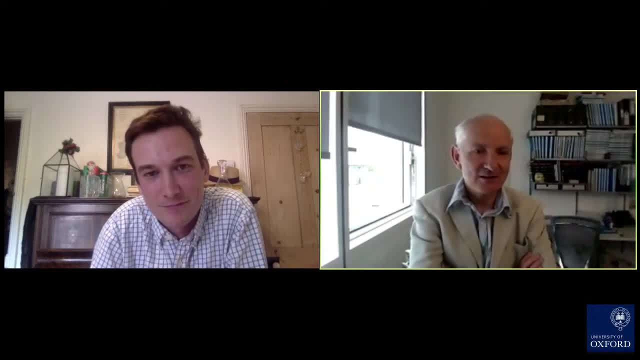 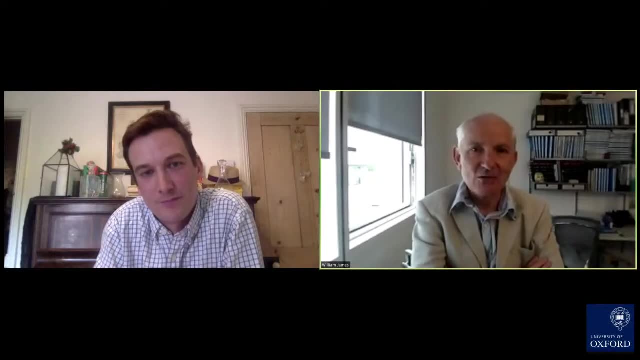 certainly learned a lot, and i think the uh, the, the questions and the viewers will have learned a great deal as well. um so um, thank you very much for that. thank you, thank all of you who've been watching this and the other covid conversations for your uh engagement. 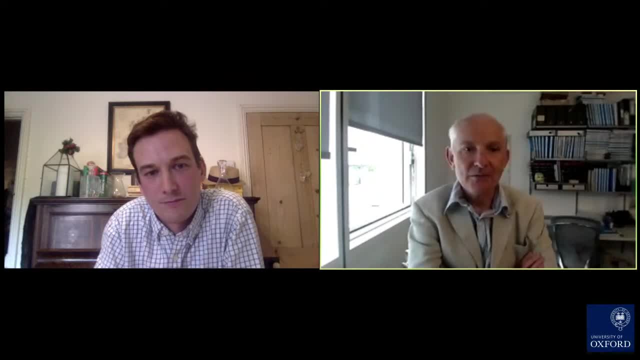 and your, your, your stimulus and your questions. um, that is the the last of this series of covid conversations. um, we've had a great time i we hope you have as well. um, i want to iterate a few points that we've made a few times in this. that that just by reviewing.